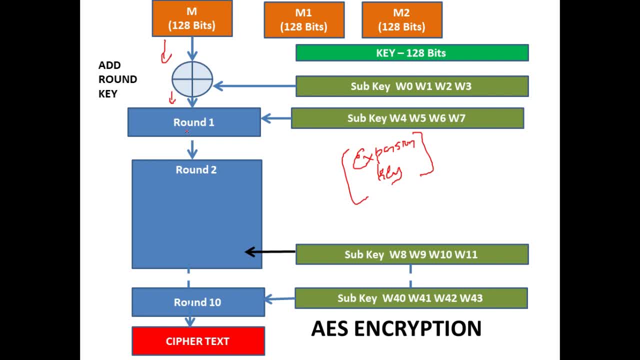 XOR it and create this input state array for a round. So now what is happening in every round is we take the state array. we have performed byte substitution. This output is given to shift rows. We'll be doing some cyclic left shift on the bytes for each row. 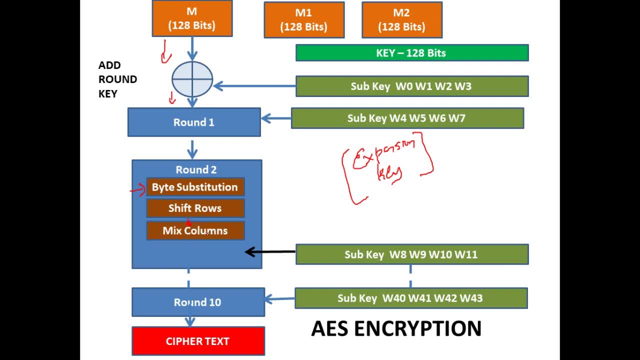 And then the output of this will be given to mix columns, wherein we'll be multiplying the state array with a standard matrix And then we'll be giving that output to add round key. Here is where we are going to use the input round key, Say for round 2, the round. 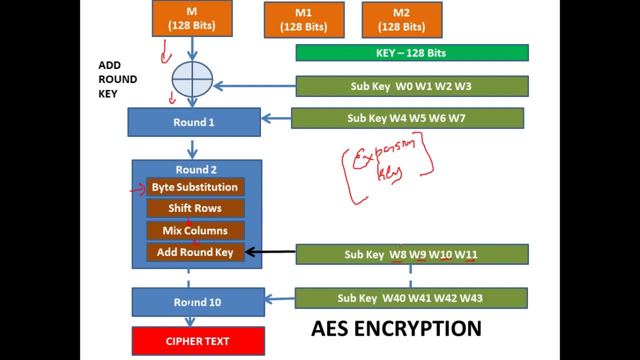 key will be word 8,, word 9,, word 10,, word 11.. So we're going to take these four words And then we are going to perform an XOR in this particular round. So this output will be given as an input to the next round. Again, this round we're going. 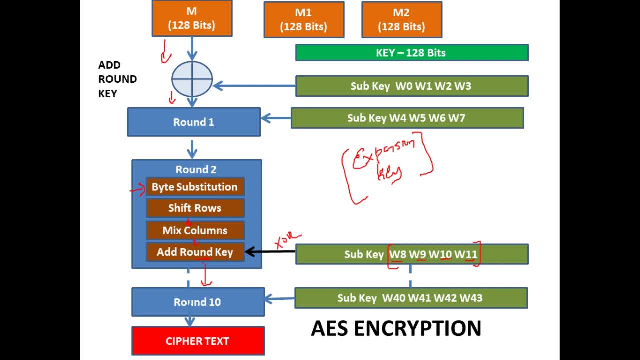 to take up all these steps: byte, substitution, shift rows, mix columns and round key. But there is only one point that we should note here: The last round, round 10, we'll not be adding the mix column step. So from round 1 to round 9, we love all of these four steps. 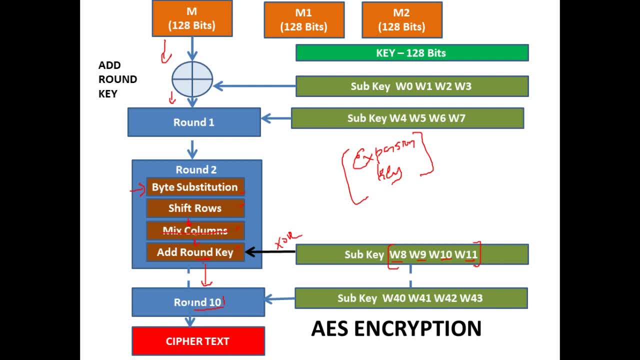 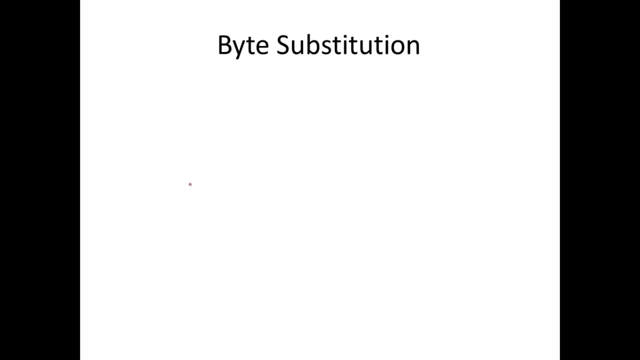 whereas only in round 10 we'll be skipping mixed columns. so we'll now take a look at every step in a round: the byte substitution step. what is byte substitution? we are going to get the state areas input to the round. we're going to take every byte substitute that with another byte. how? 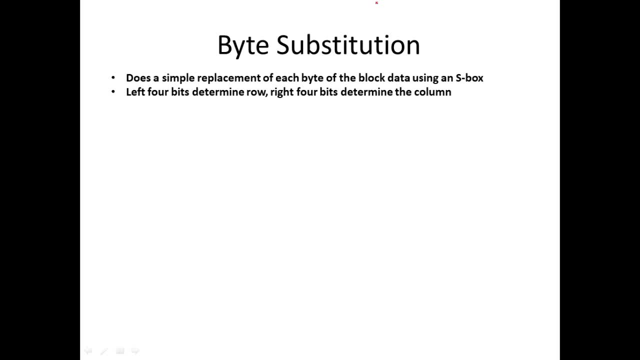 will you substitute for that? you will use an S box, so let us understand this here. so this is the input after we perform an XOR of the subkey 0 with the input message: you're going to get this right. this is input to our round 1. 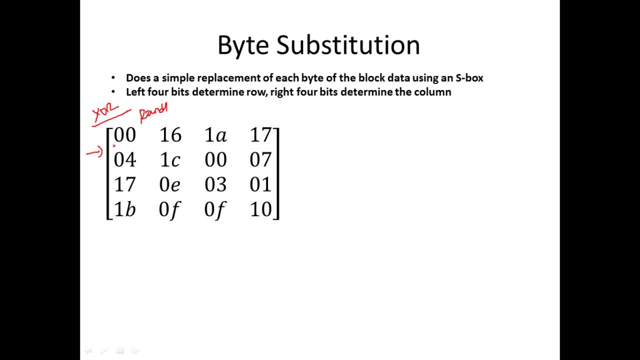 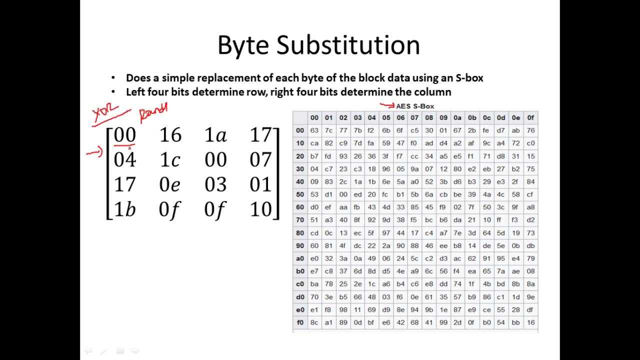 and what we are going to do here is byte substitution, that is, take every byte and substitute that with another byte. for that we'll use this S box. so 0, 0. so here 0 is for the rows and this 0 is for the column. so 0 is for the rows and this 0 is for the column. so 0 is for the rows and this 0 is for the column. so what is 0 0? we'll substitute 0 0 as. so what is 0 0? we'll substitute 0 0 as. 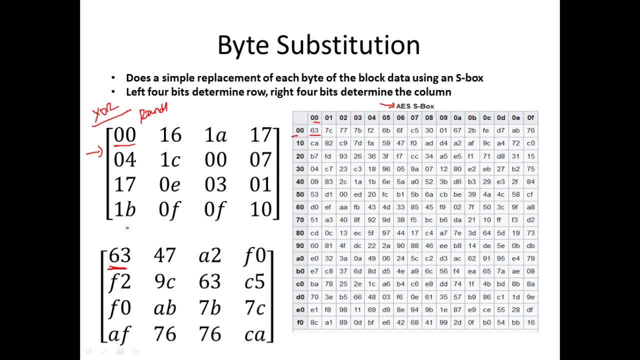 so what is 0: 0? we'll substitute 0: 0 as 63 in our output, 63 in our output, 63 in our output, so that is byte substitution. take a byte, so that is byte substitution. take a byte, so that is byte substitution. take a byte, substitute that with another byte for. 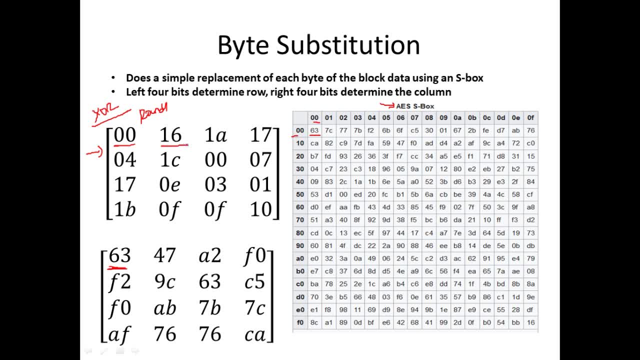 substitute that with another byte for. substitute that with another byte for that use this S box. that use this S box. that use this S box. so 1: 6 how it is getting changed, you go. so 1: 6 how it is getting changed, you go. 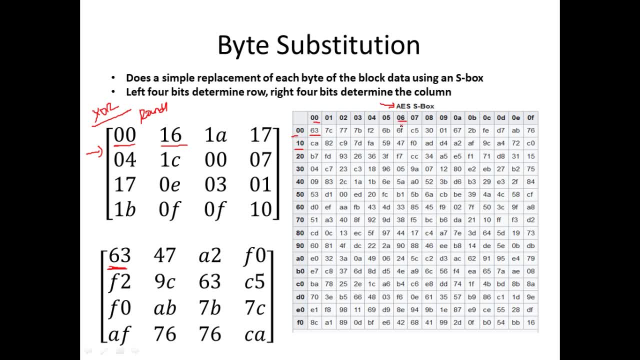 so 1, 6, how it is getting changed. you go to 1 year and where is 6? 6 is here. what to 1 year? and where is 6? 6 is here. what to 1 year and where is 6? 6 is here. what is the intersection of 1 and 6- 47? so 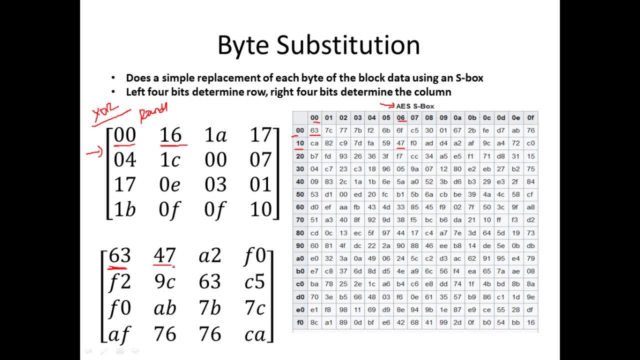 is the intersection of 1 and 6: 47. so is the intersection of 1 and 6: 47. so you're going to substitute 1- 6 as 47 in. you're going to substitute 1- 6 as 47 in. you're going to substitute 1- 6 as 47 in the output. so what is 1 a? so this is 1. 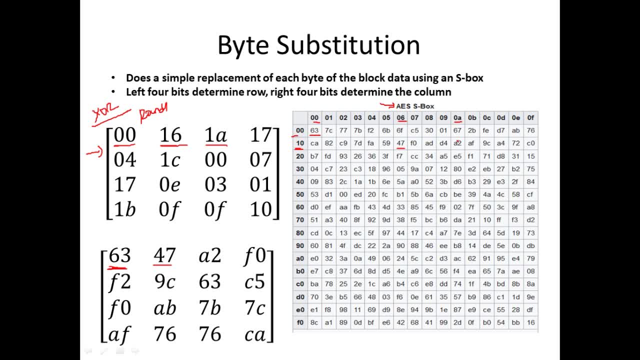 the output. so what is 1 a? so this is 1 the output. so what is 1 a? so this is 1. and where is a a is here, so what is this? and where is a a is here? so what is this? and where is a a is here, so what is this? this is a 2, so 1 a is getting substituted. 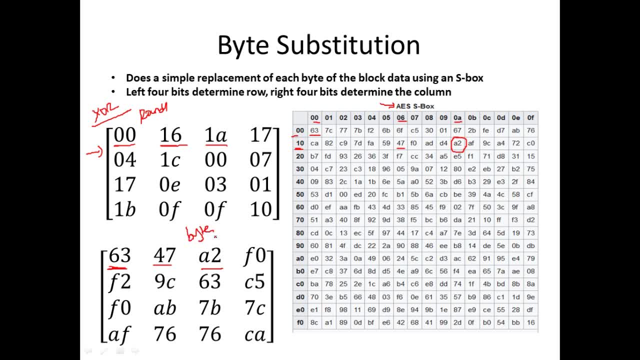 this is a 2, so 1 a is getting substituted. this is a 2, so 1 a is getting substituted as a 2, so this step is called byte as a 2. so this step is called byte as a 2, so this step is called byte substitution. 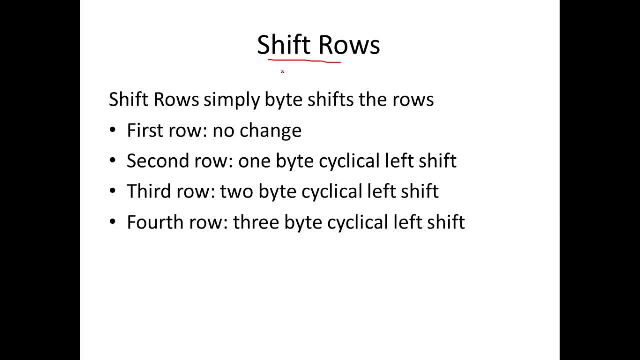 the next step is. the next step is the next step is shifting, shifting, shifting, shifting rows. so after you finish bite rows, so after you finish bite rows, so after you finish bite, substitution. this will be our input to substitution, this will be our input to substitution, this will be our input to the next step, that is, shift rows. 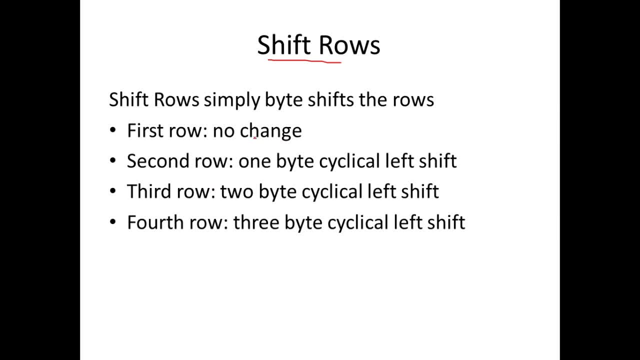 the next step, that is shift rows. the next step, that is shift rows. what shift rows does is all. what shift rows does is all. what shift rows does is all: a circular left shift, a circular left shift, a circular left shift. so the we are going to take the first. 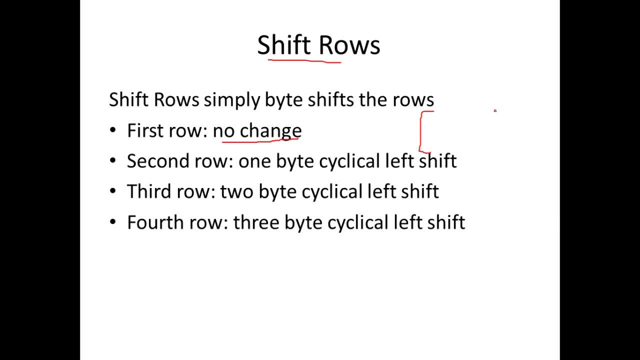 so the we are going to take the first. so the we are going to take the first row. we are not going to do any change. row. we are not going to do any change row. we are not going to do any change. so our input is a 4 cross, 4 matrix. 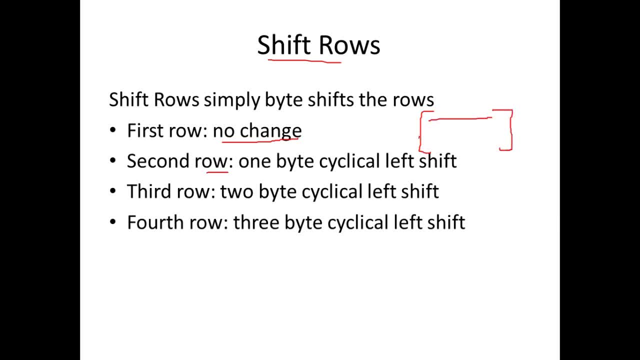 so our input is a 4 cross 4 matrix. so our input is a 4 cross 4 matrix. the first row: we are not going to do any. the first row. we are not going to do any. change, change, change. the second row will take the second row. 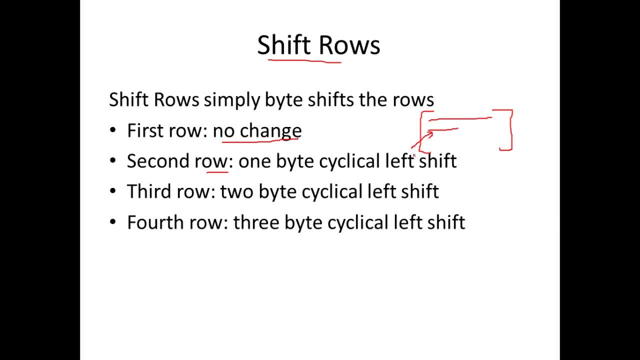 the second row will take the second row. the second row will take the second row. perform a, perform a. perform a. circular left shift of one byte. likewise, circular left shift of one byte. likewise, circular left shift of one byte. likewise. you take third row. that is the third row. 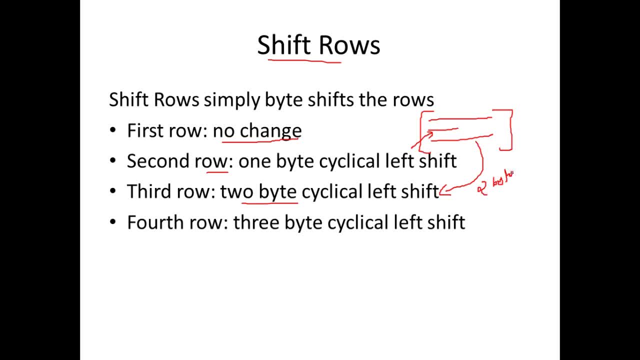 you take third row, that is the third row. you take third row, that is the third row. and then we'll do a circular left shift, and then we'll do a circular left shift, and then we'll do a circular left shift of two bytes, of two bytes. 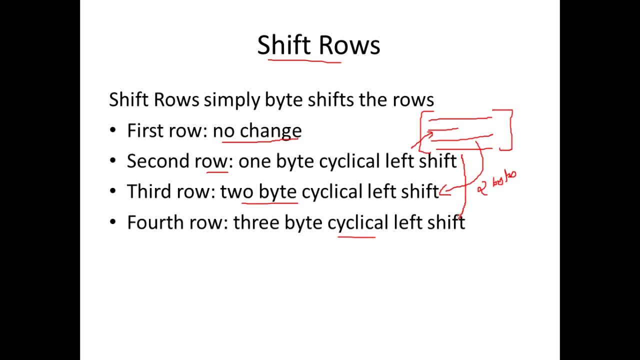 of two bytes. likewise, we take fourth row. this is the likewise. we take fourth row. this is the likewise. we take fourth row. this is the fourth row. fourth row, fourth row, and what we'll do is we'll do a circular, and what we'll do is we'll do a circular. 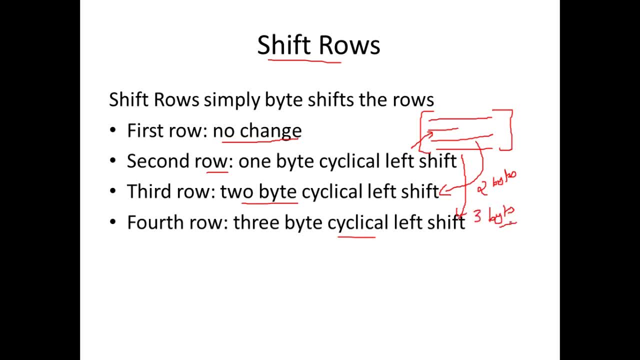 and what we'll do is we'll do a circular left shift of three bytes. so we'll see that with the input that. so we'll see that with the input that. so we'll see that, with the input that we are receiving, we are receiving, we are receiving, say, this is the input that we have. 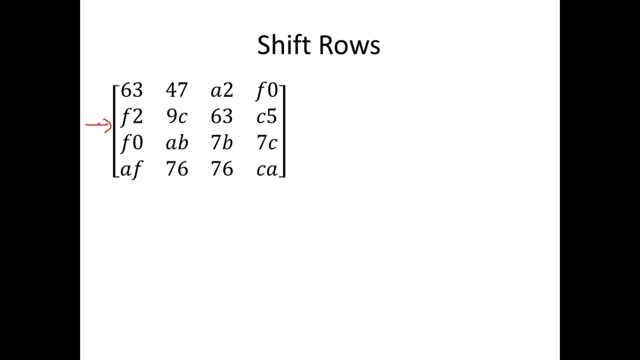 say this is the input that we have, say this is the input that we have achieved after our byte substitution step achieved after our byte substitution step achieved after our byte substitution step in a particular round round one. let's say in a particular round round one. let's say: 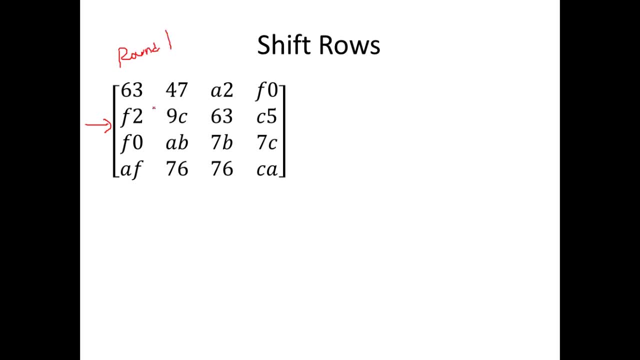 in a particular round, round one, let's say in round one, in round one, in round one, after byte substitution is over. this is after byte substitution is over. this is after byte substitution is over. this is our input to our input, to our input to shift rows. so we are not going to do. 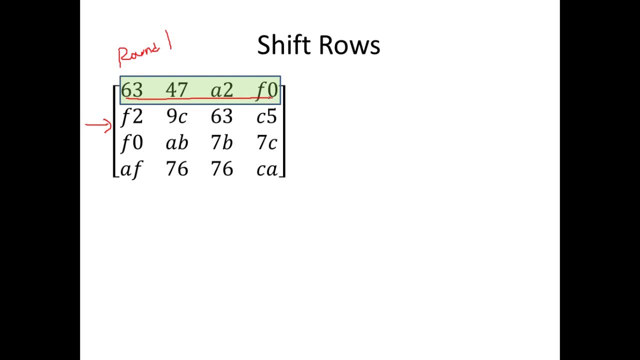 shift rows. so we are not going to do shift rows. so we are not going to do anything to the first row. there is no anything to the first row. there is no anything to the first row. there is no change. we're going to leave it like that. 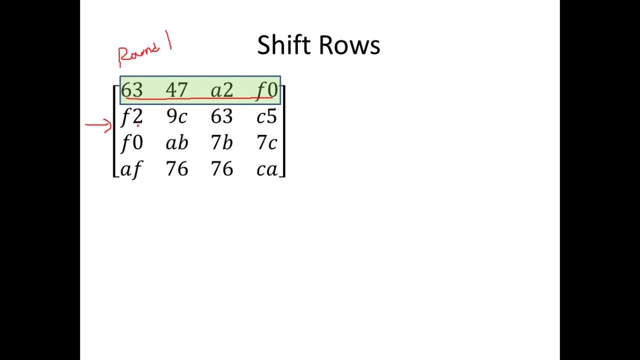 change. we're going to leave it like that change. we're going to leave it like that. whereas we're going to take the second, whereas we're going to take the second, whereas we're going to take the second row, we'll do a circular left shift by. 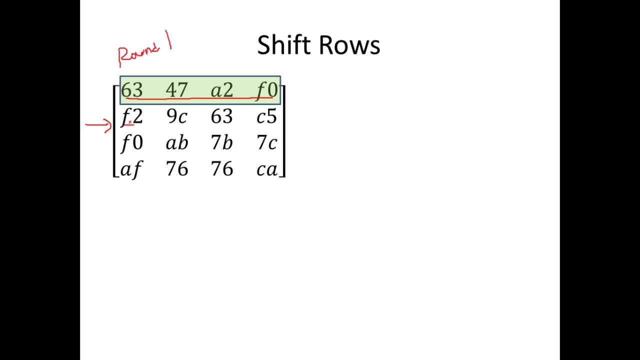 row. we'll do a circular left shift by row. we'll do a circular left shift by one byte. that is what does that mean. one byte, that is what does that mean. one byte. that is what does that mean. we're going to take f2, move this f2 to. 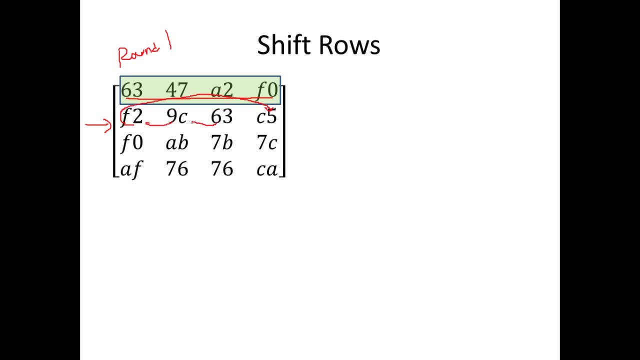 we're going to take f2, move this f2 to. we're going to take f2, move this f2 to the end, the end, the end. and we'll push everything to the left by, and we'll push everything to the left by and we'll push everything to the left by one step. say, you see, a 9c has come. 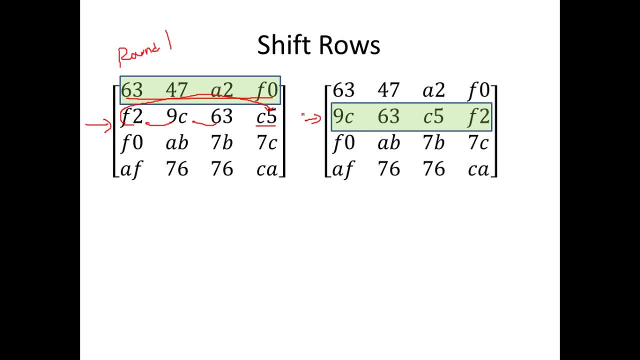 one step say: you see a 9c has come. one step say: you see a 9c has come. front: 9c63 c5: this f2 has been pushed to front. 9c63 c5: this f2 has been pushed to front. 9c63 c5: this f2 has been pushed to the end. 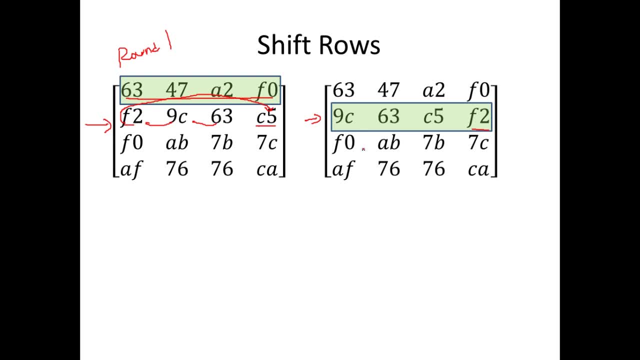 what is the next step? and we do a. what is the next step? and we do a. what is the next step? and we do a circular left shift by two bytes. that is circular left shift by two bytes. that is circular left shift by two bytes. that is, we push f0 and ab to the end and push. 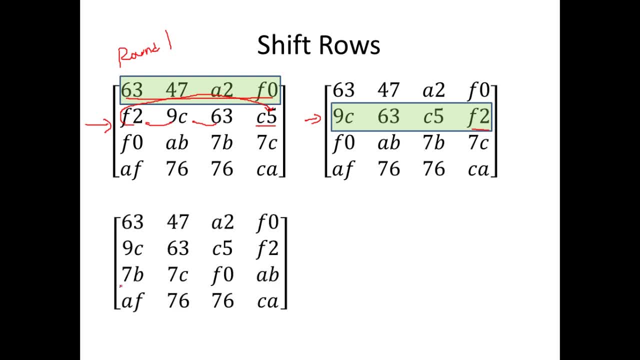 we push f0 and ab to the end and push, we push f0 and ab to the end and push 7b and 7c to the front, 7b and 7c to the front, 7b and 7c to the front. so this is row 3 and we take row 3 and 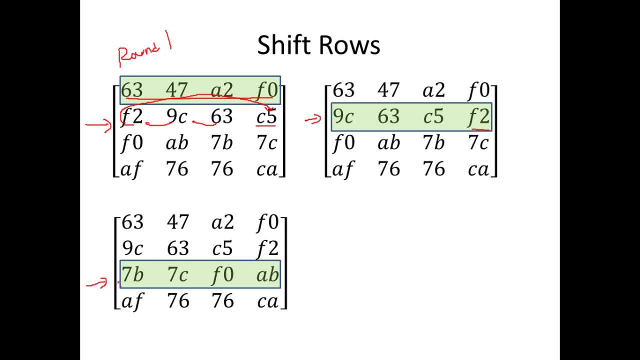 so this is row 3 and we take row 3. and so this is row 3 and we take row 3 and perform a circular left shift by two. perform a circular left shift by two. perform a circular left shift by two, bytes, bytes, bytes. after this, we go to row 4 and we're 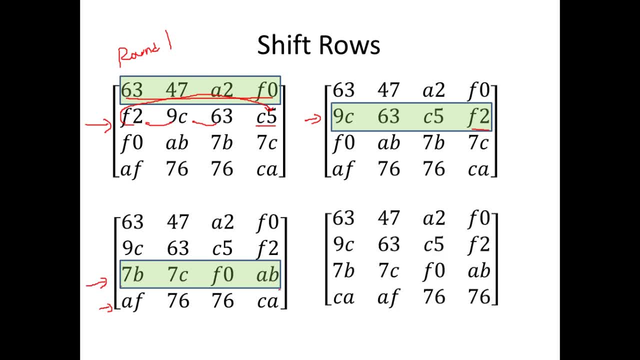 after this, we go to row 4 and we're after this, we go to row 4 and we're going to take the three bytes and do a going to take the three bytes and do a going to take the three bytes and do a circular left shift. so what will be the? 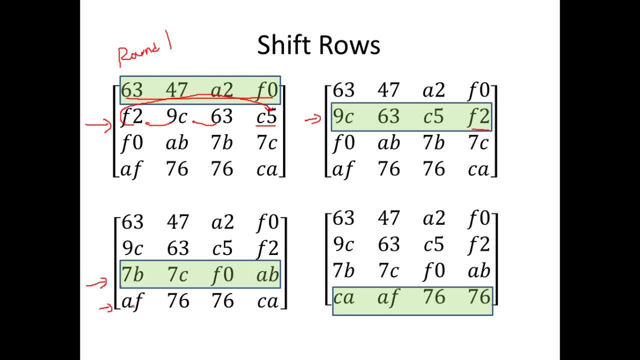 circular left shift. so what will be the circular left shift? so what will be the output here? you see here output here. you see here output here. you see here the first three bytes, so af the first three bytes, so af the first three bytes, so af 76, 76 is pushed to the end and ca. 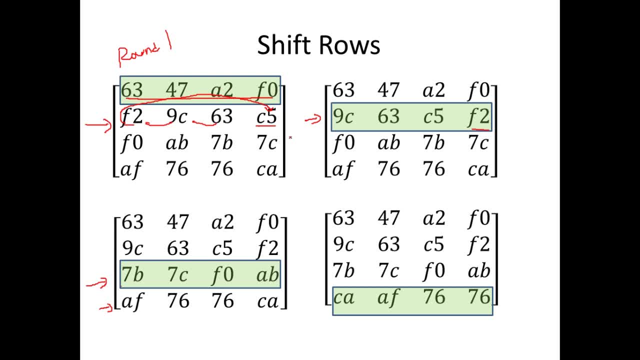 the first three bytes, so af 76- 76 is pushed to the end. and ca: the first three bytes, so af 76- 76 is pushed to the end. and ca: circular left shift by one byte. circular left shift by one byte. circular left shift by one byte. third row: circular left shift by two. 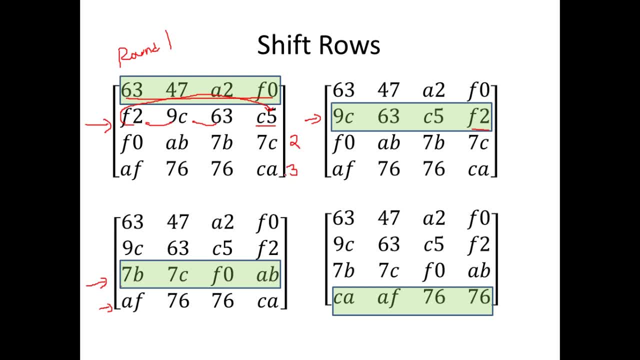 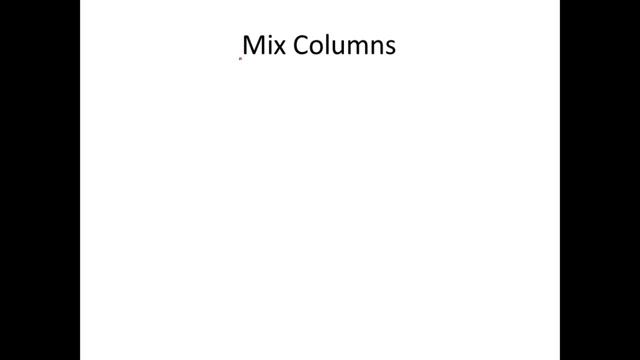 third row, circular left- shift by two. third row, circular left- shift by two bytes. fourth row, circular left- shift by bytes. fourth row, circular left- shift by bytes. fourth row, circular left- shift by three bytes. after we shift all the rows the next. after we shift all the rows, the next. 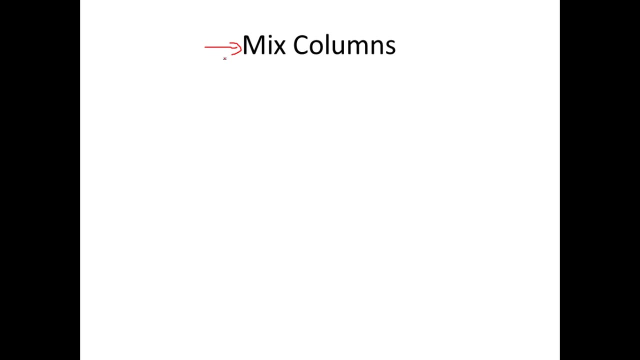 after we shift all the rows, the next step that comes in a round is mix. step that comes in a round is mix step that comes in a round is mix: columns, columns, columns. so this is the output we achieve after. so this is the output we achieve after. 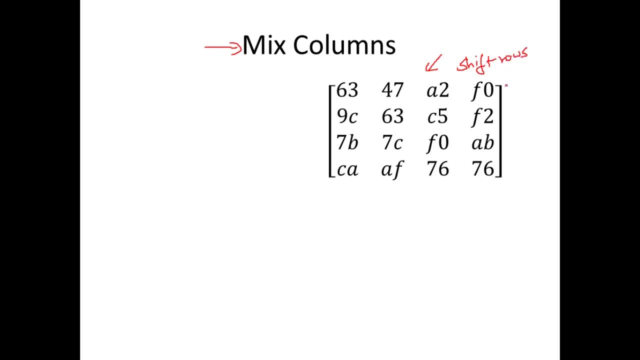 so this is the output we achieve after our shift rows, our shift rows, our shift rows in round one, in round one, in round one. to do is we need to take this and to do is we need to take this and to do is we need to take this and multiply that. 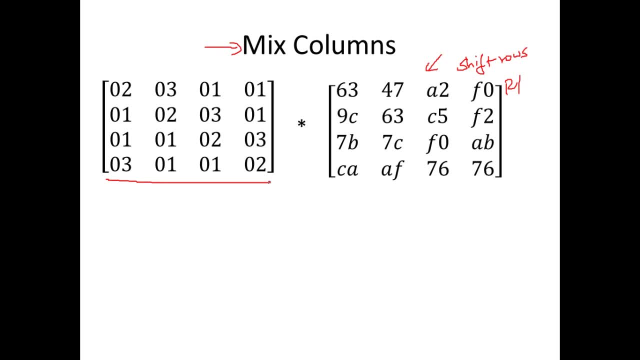 multiply that. multiply that with another matrix. so this is a standard with another matrix. so this is a standard with another matrix. so this is a standard matrix, matrix, matrix. we are going to use and we are going to. we are going to use and we are going to. 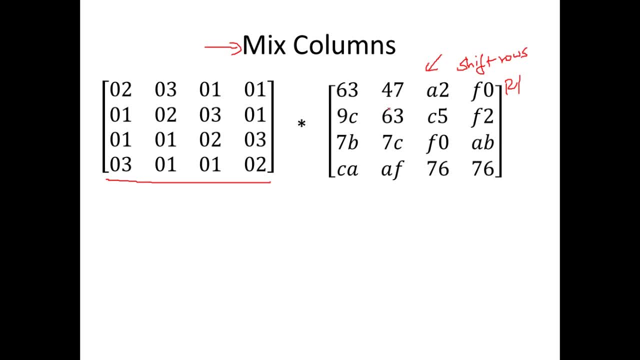 we are going to use and we are going to multiply, multiply, multiply this result that we have achieved from our, this result that we have achieved from our, this result that we have achieved from our shift rows, shift rows, shift rows, with this matrix in mixed columns, with this matrix in mixed columns. 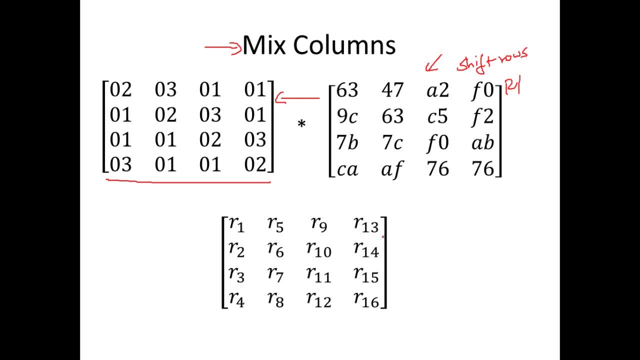 with this matrix in mixed columns, the result after multiplication will be the result after multiplication will be the result after multiplication will be another, another, another state array or 4 cross 4 matrix. that state array or 4 cross 4 matrix. that state array or 4 cross 4 matrix that is given here: r1, r2, r3, r4, r5, r6, r7. 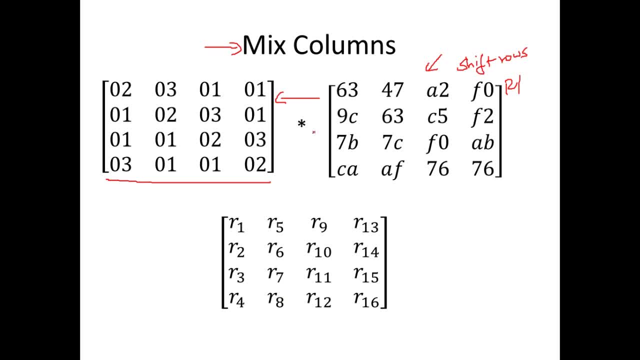 is given here: r1, r2, r3, r4, r5, r6, r7. is given here: r1, r2, r3, r4, r5, r6, r7, r8. so that is the mixed column step. so how? so that is the mixed column step. so how? 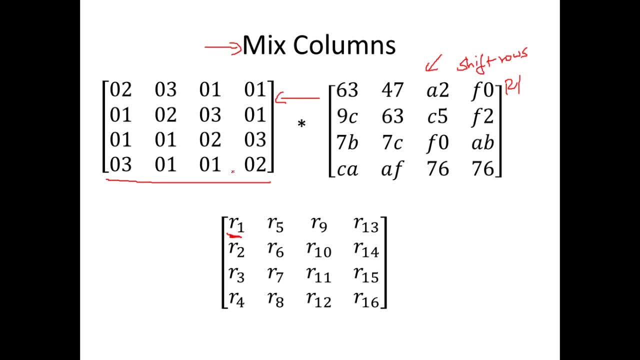 so that is the mixed column step. so how will you? will you? will you determine r1? how can we determine r1 if determine r1? how can we determine r1 if determine r1? how can we determine r1 if these are the two matrices? these are the two matrices. 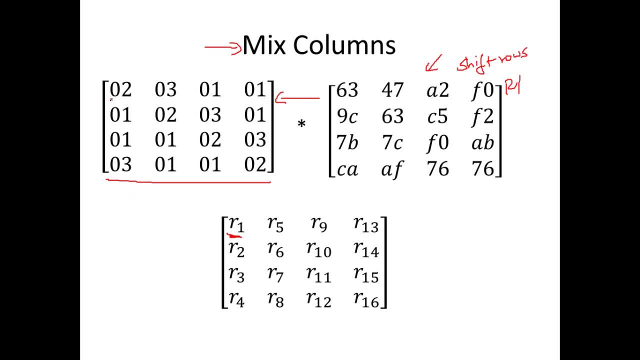 these are the two matrices. how will you perform that it is nothing? how will you perform that it is nothing? how will you perform that it is nothing but but? but you take this row, you take this row, and then you multiply that with this, and then you multiply that with this. 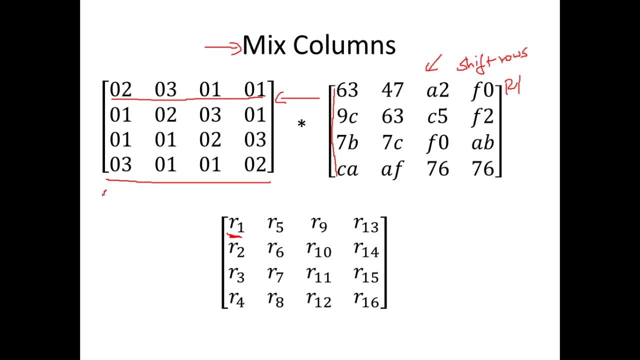 and then you multiply that with this column, column, column. so what is r1 here, that is 0, 2. so what is r1 here, that is 0, 2. so what is r1 here, that is 0, 2, into 63 plus plus. 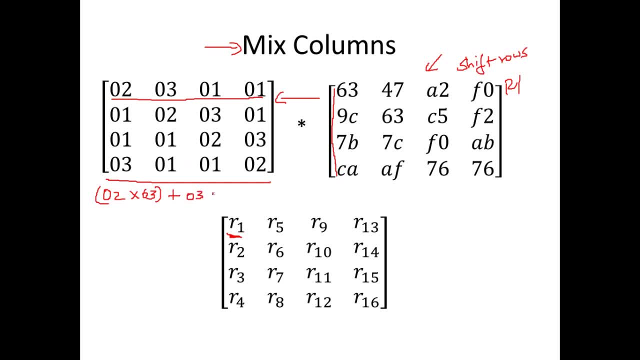 plus 0, 3 into 9c. plus plus plus 0, 1 into 7b, 0, 1 into 7b, 0, 1 into 7b, plus this 0, 1 into ca. so this result is nothing but r1. 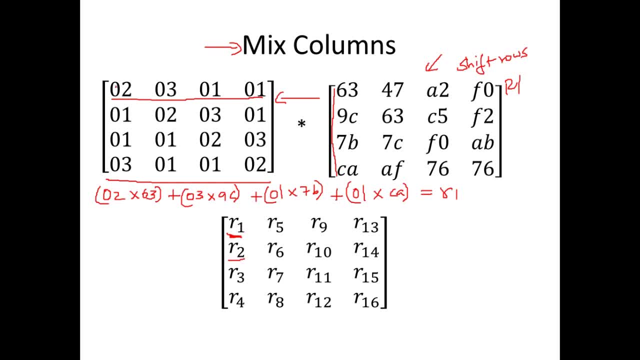 likewise, how will you find r2? likewise, how will you find r2? likewise, how will you find r2? you take this row 2, you take this row 2, you take this row 2, and then you multiply that with, and then you multiply that with. 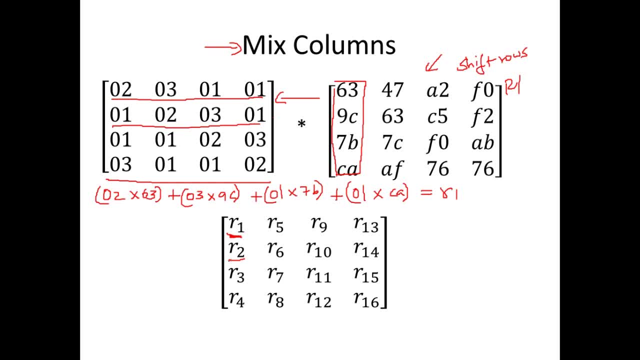 and then you multiply that with this column, this column, this column, that will lead to R2.. Can we write the equation for R2?? It is nothing but 0, 1 into 63.. 0, 2 plus simple matrix multiplication: 0, 2 into 9C plus 0, 3 into 7B plus 0, 1 into CA. What is this? 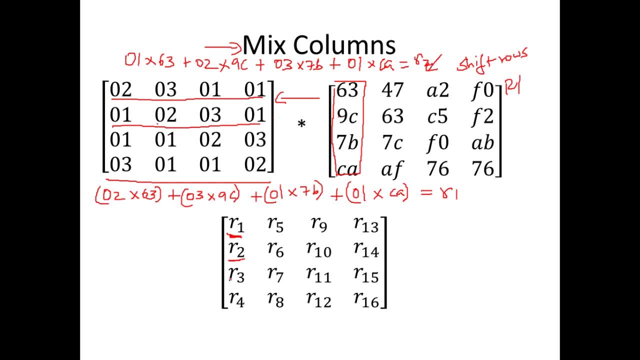 This is R2 in our result. If you want to find R3, what are you going to do? You are going to take this row 3, multiply that with 63,, 9C, 7B, CA. You are going to get R3.. So you. 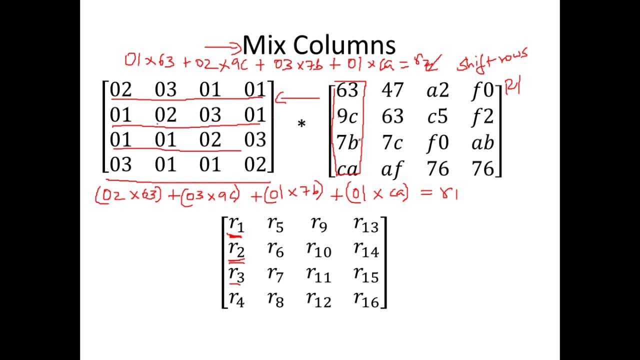 repeat these steps to complete your output. So this is where the concept of Galois field is coming to place. So whatever multiplication and addition you are doing here, that is with respect to a Galois field, So finite field arithmetic is used here. It is not just ordinary. 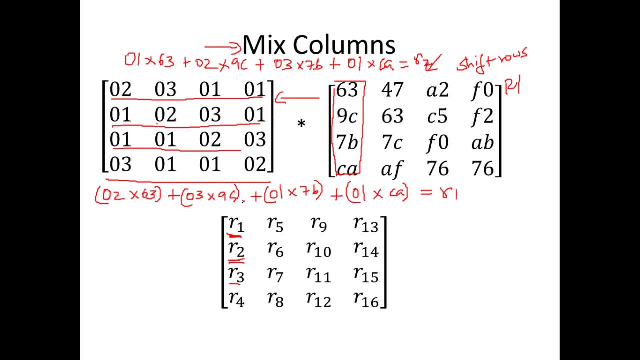 multiplication or addition. It is finite field arithmetic that is used here. So let us see what is this: 0, 2 into 63.. How it is done. What is the result that we are achieving here? So finite field arithmetic comes into play. 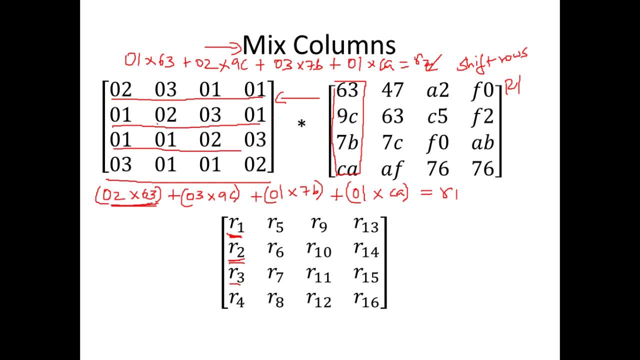 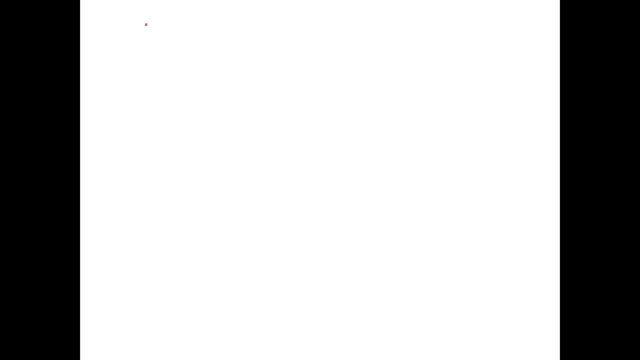 We will see how to get the result of 0, 2 into 63. Then you will understand how we are using finite field arithmetic here. What we have here is 0, 2.. 0, 2 is represented as, say, these are hexadecimal characters, So in binary it is nothing but 0,, 0 and 2 is 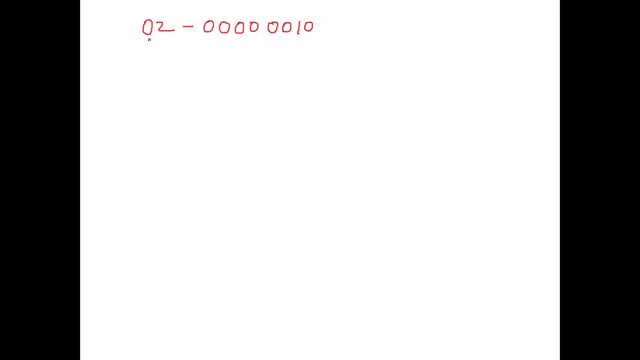 represented as 0, 0, 1, 0.. So since these are hexadecimal, we convert that to binary. And these: 8,, 10,, 11,, 12,, 13,, 14,, 15,, 16,, 17,, 18,, 19,, 20,, 21,, 22,, 23,, 24,, 25,, 26,, 27,, 28,, 29,, 30,. 30,, 31,, 32,, 33,, 34,, 35,, 36,, 37,, 38,, 38,, 39,, 40,, 42,, 43,, 44,, 45,, 46,, 47,, 49,, 40,, 41,, 42,, 43,. 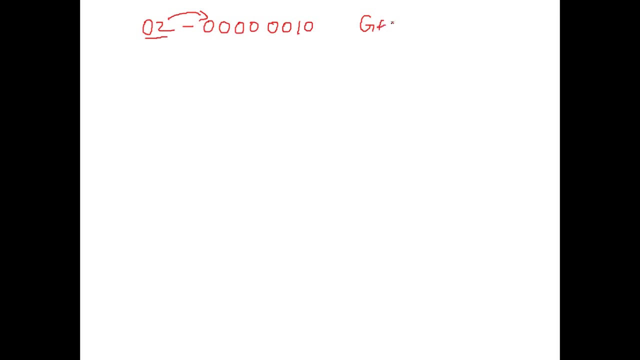 45,, 48,, 49,, 42,, 43,, 44,, 45,, 46,, 47,, 49,, 42,, 44,, 45.. actually represent a polynomial in G of 2 for 8.. 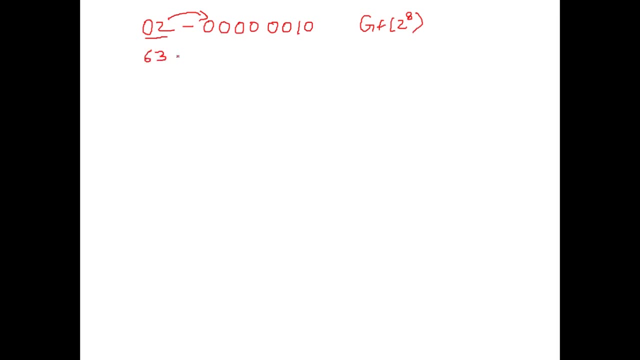 Likewise, what is the next number? 63 is an hexadecimal. What is the representation of 63?? 6 is represented as 0, 1, 1, 0.. This is for 6, and 3 is represented as 0, 0,, 1, 1.. 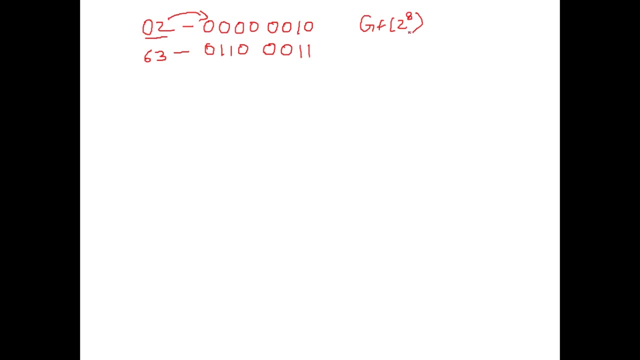 So again, this is a polynomial in GF 2, power 8. so can we go and write the corresponding polynomials for 0, 2 and 63. what is 0, 2? the polynomial will be. it's actually a polynomial in GF 2. 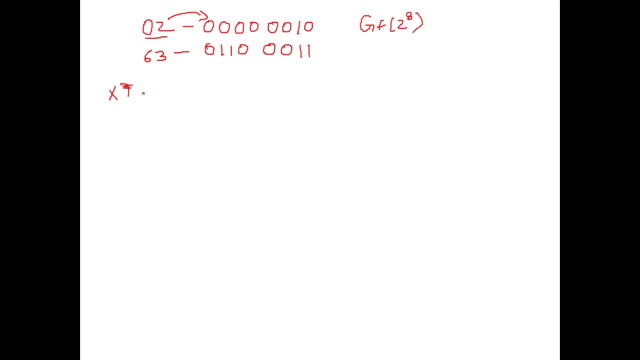 power 8 takes the form: X power 7 plus X power 6 plus X power 5 plus X power 4 plus X for 3 plus X for 2 plus X plus 1. since all the bits are zeros here, there is only one here, so you're going to just have this one term and everything else. 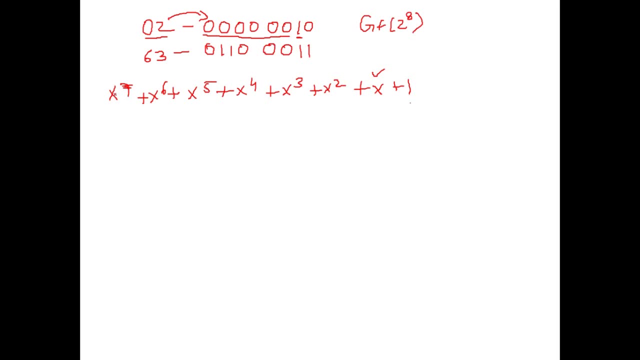 is going to be 0, so this is 0, 0, 0, 0, 0. so, since all of these things are zeros, so what is the element we have here? the polynomial corresponding to 0, 2 is X, so 0, 2 is represented as X, a polynomial. 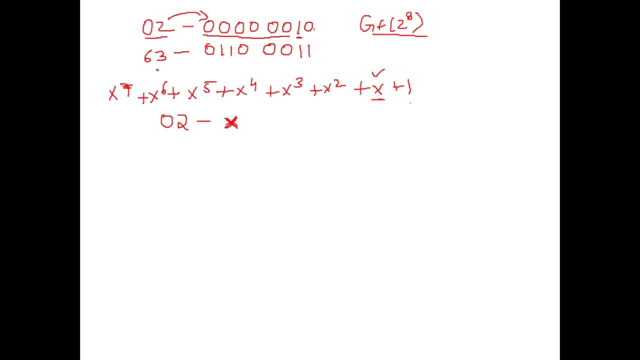 X in GF 2, power 8, likewise 63. what are the terms in 63? so we can write it here: X power 7 is 0. so we have X power 6 and we have X power 5. this is 0. this is that. 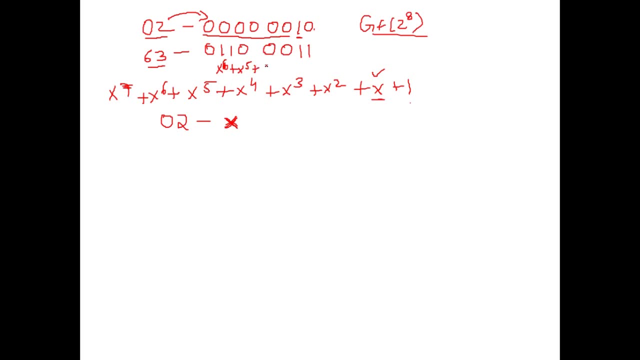 is X. power 4 is 0, X power 3 is 0, X power 2 is 0. we have X and we have plus 1, so this is the polynomial corresponding to 63 in GF 2, par 8. so we have two polynomials. now what are those two? 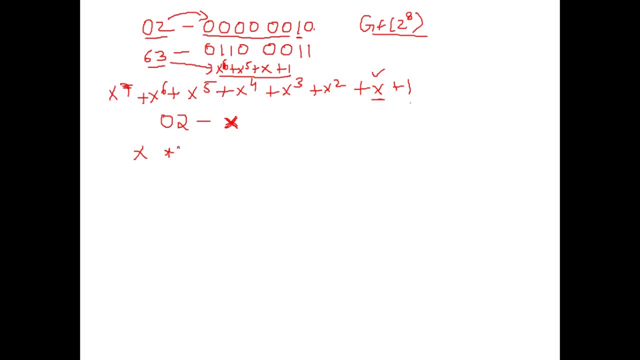 polynomials. one is an X and that should be multiplied with another polynomial, that is this: X power 6 plus X power, 5 plus X plus 1. so let's go and multiply these two polynomials, so we'll multiply X. so it's nothing but X for 7 plus X, 4, 6 plus X, square plus X. so this is. 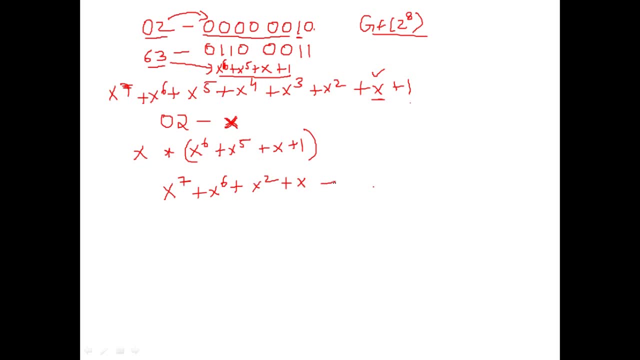 the result of the multiplication. so how will you represent this polynomial in binary? it is nothing but x power. 7 is there? x power? 6 is there? x power 5 is missing, 4 is missing, 3 is missing. we have x square and we have x, whereas 1 is missing, and this can be converted to x. take the four bits you write. 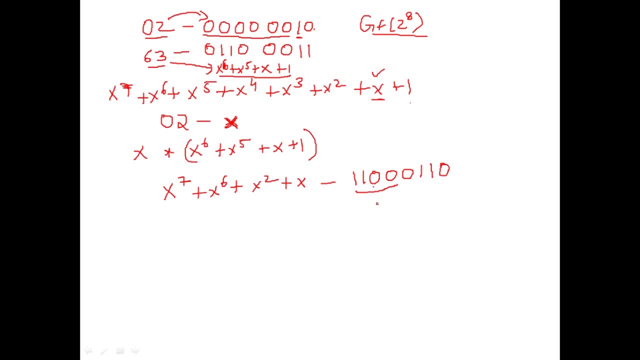 the x representation. so this is 12. 12 in hexadecimal is c and this is 0, 1, 1, 0. that is nothing but 6.. so the result of multiplying 0, 2 into 63 is nothing but c, 6. so here the concept. 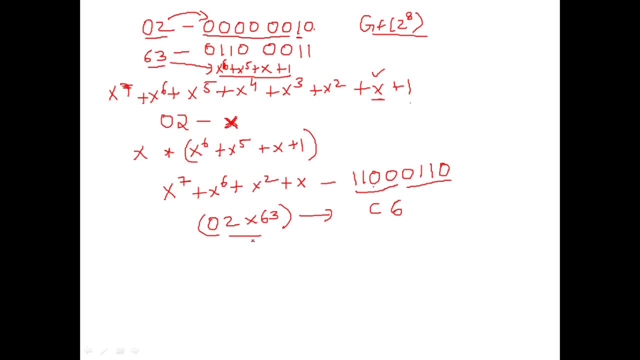 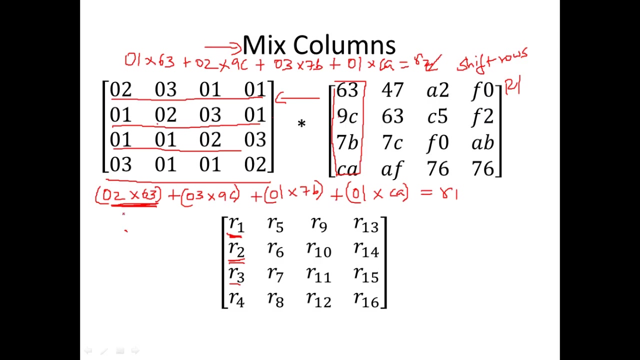 we are going to use is finite field multiplication. so every operation we do inside this matrix is a finite field arithmetic. please have this in mind. so we have found out what is the answer to 0, 2 into 63 using finite field. that is nothing but c, 6, like that we should compute everything. 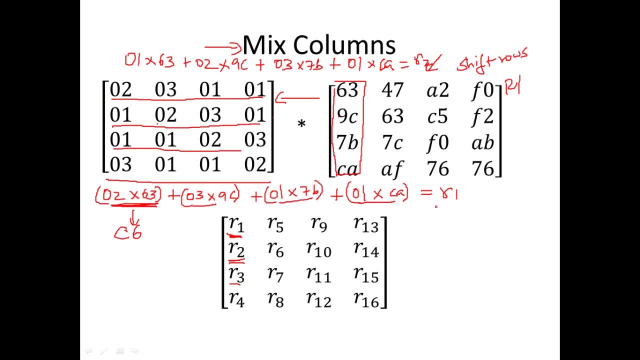 convert that to a polynomial, perform the multiplication and finally attain what is r1. like that we can compute r2, r3 by completing this multiplication. so i'm not going to go into the details of the multiplication, but i'm going to go into the details of the multiplication. so i'm not going to go into the details of the multiplication, so i'm not. 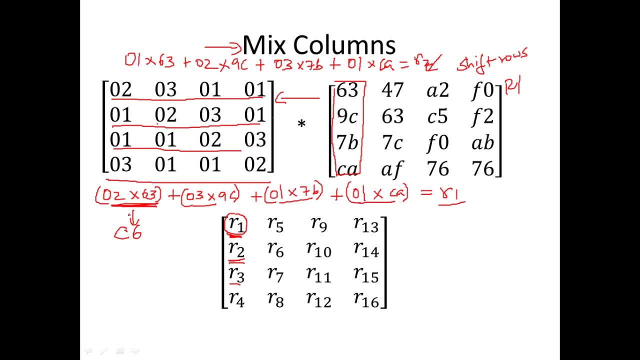 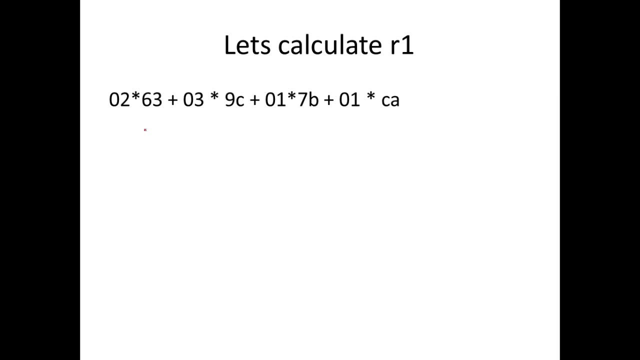 going to go over everything. i know how difficult it is. i'll just tell you how to compute this entire term. we'll wind up mixing columns, understanding by computing r1. so let's compute r1. what is that? it is nothing but 0, 2 into 63 plus 0, 3 into 9 c plus 0, 1 into 7 b. 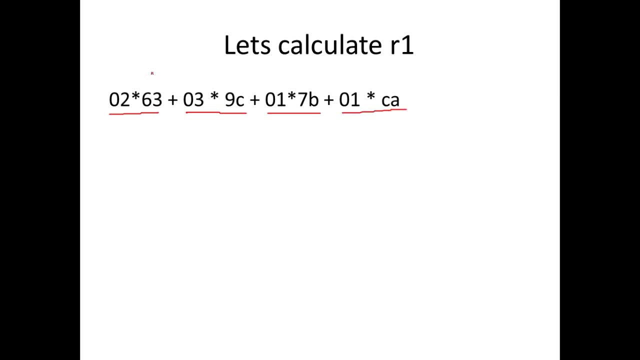 plus 0, 1 into c a. we already computed 0, 2 into 63, but this is another easy way of computing this value for r1. so we represent 0, 2 in binary. it is 0, 0, 0, 0. 2 is 0, 0, 1, 0 this entire term. 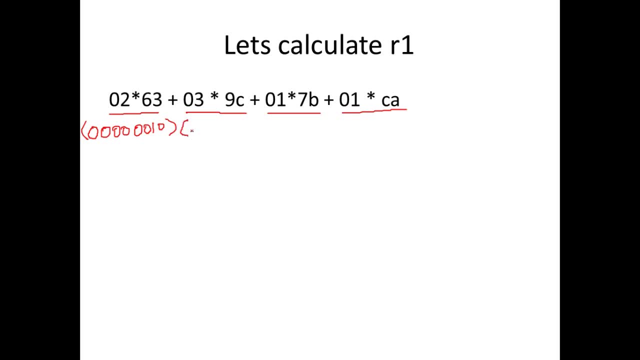 should be multiplied with 63. what is 63? that is nothing but 0, 1, 1, 0, and 3 is 0, 0, 1, 1, so this has been represented, and plus what is 0, 3, so this 3 is nothing but zero, zero. 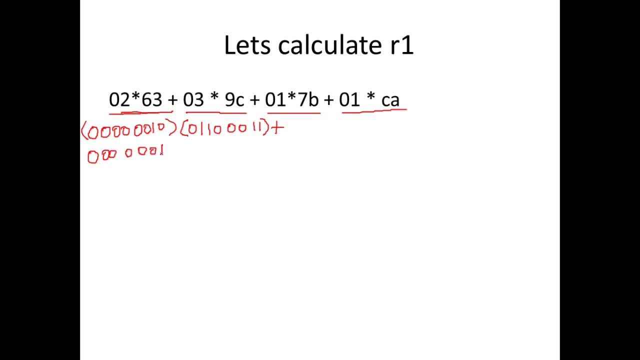 zero, zero, and then zero, zero, one, one. so this is zero. three into nine c what is nine? that is one zero, zero one. four bits for representing nine. c is twelve, that is one one, zero, zero. plus what is zero, one, zero, one, zero. first, four bits are zeros. next four bits represent a one. 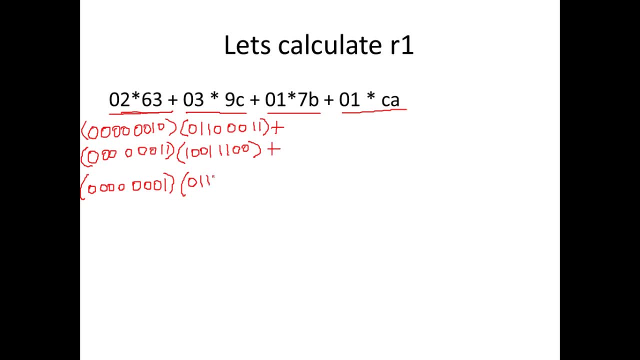 what is seven b, seven is nothing but zero, one, one one. what is b, b is eleven, so it is eight, zero one one. so this is seven, b plus again zero one. so what is zero, zero, zero, zero and zero, zero, zero one. this is, this is actually zero one. and what is c? c is a twelve, right, one, one, zero, zero. 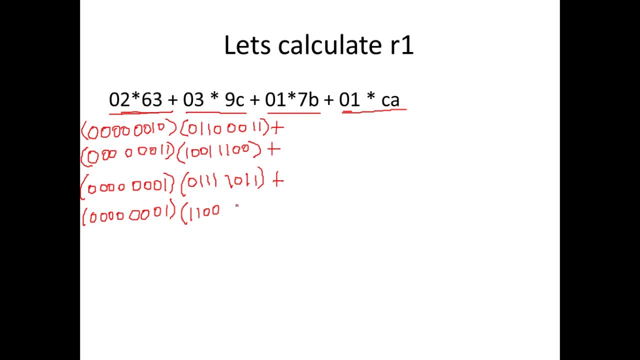 that is the binary representation of c, and what is a a is a ten. so it should be one zero, one zero. so now we can convert this to polynomials. uh, can we write the corresponding polynomials? so all the terms are zero except for an x. so that is x. into what are the terms here? so we have x power 6, x power 5. 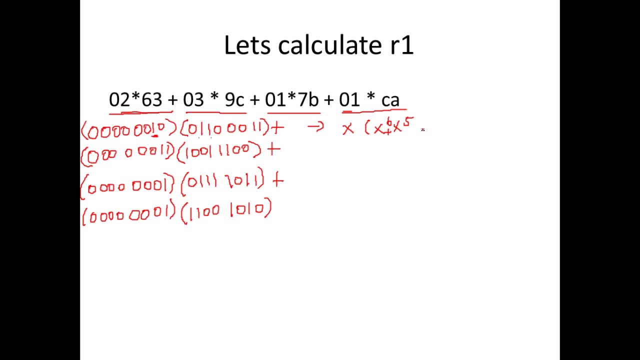 the x power 7 is 0, so we have x power 6, x power 5 plus x power, 4, x power 3, x power 2 is a 0, so we love x plus 1. so this is the corresponding polynomial representation of these two. 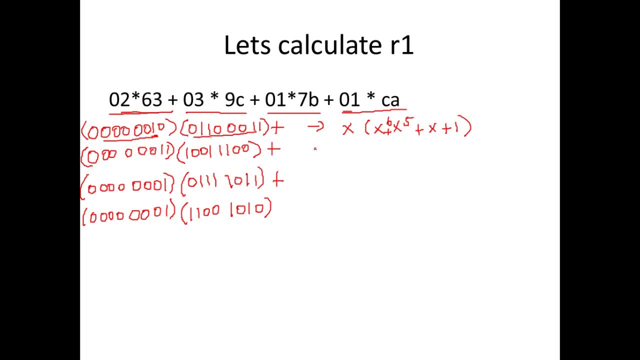 uh binary elements in g of 2 power 8. likewise we can also perform an addition right x into x power 6 plus x, power 5 plus x plus 1, plus. again we go and represent this in polynomial. we have only two terms, x and 1, so it is x plus 1. into what is the polynomial representation of this? we have x. 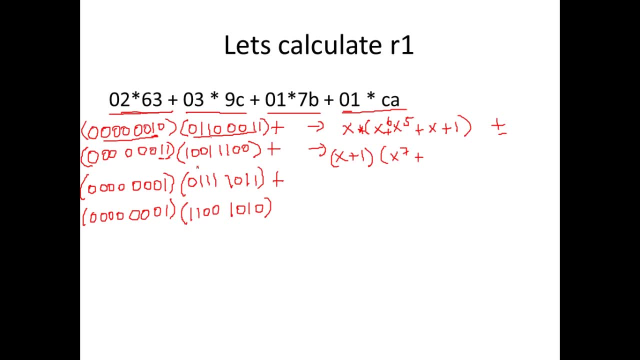 power 7 plus x power 6 and x power 5 are zeros. so we have x power 4 plus x power 3 plus x square x and 1 or 0, so we leave that plus. how will you represent this in polynomial, so you? 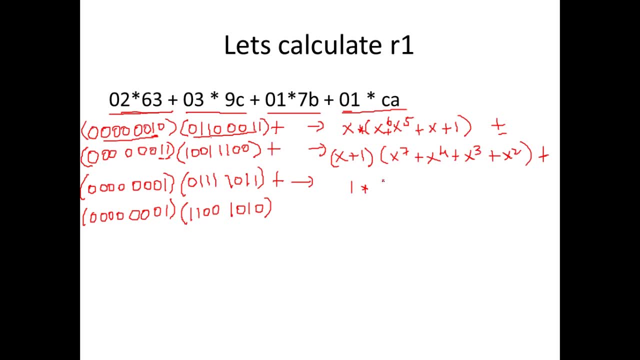 have just a 1, so it's just 1 star. what is this entire thing? so x power 7 is 0, so you have x power 6 plus x power 5 plus x power 4 plus x power 3 plus x power 4 plus x power 3 plus x power 3 plus x power 3. 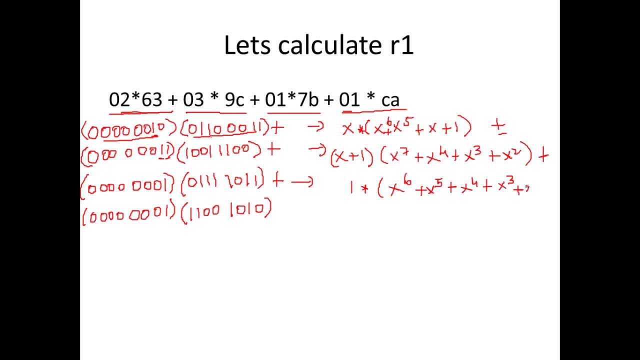 plus x power 4 plus x power 3 plus x power 3 plus x power 4 plus x power 3 plus x power 3 plus x power 3: x square is 0, so you have plus x plus 1. that's what i have given there. x power 7 is 0, so x power 6 plus x power 5 plus x power 4 plus x. 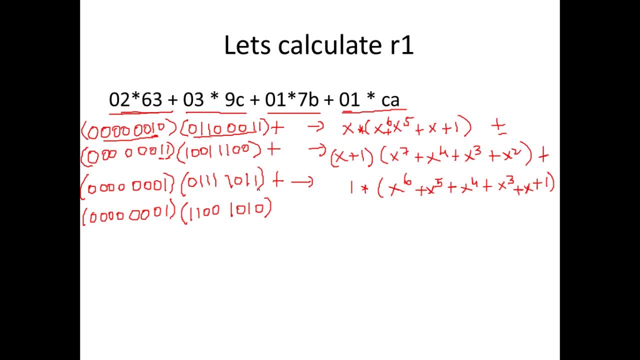 power 3. x square is 0, so x x plus 1 remains. likewise, this term will do a plus with this. what is this? this is nothing but one one into what are the terms here? x power 7 plus. x power 6 plus. so we have 5 4, 0, so we have x power 3 remaining. 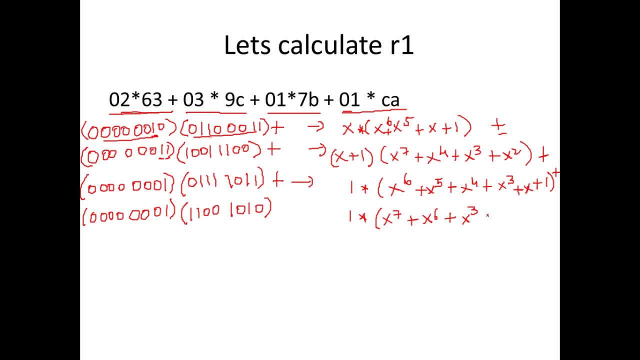 and this is a 0, x square is a 0 and we have x. okay, so we have converted that to binary. represent that in polynomial terms. okay, now let us multiply all these polynomials. so let's take x and multiply with this term, but it is nothing but x power 7 plus x power 6 plus x squared. 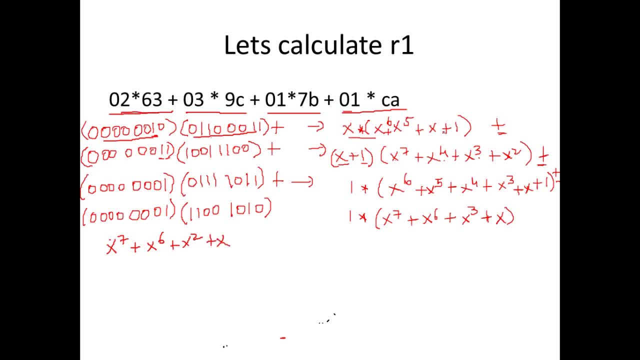 plus x. we have finished multiplying x with this term, so there is a plus here. plus now we'll multiply x with this term. so what is that? that is nothing but x power 8 plus x for f, i plus x power 4 plus x power 3. so if we finished multiplying x with this term, plus there is a 1. 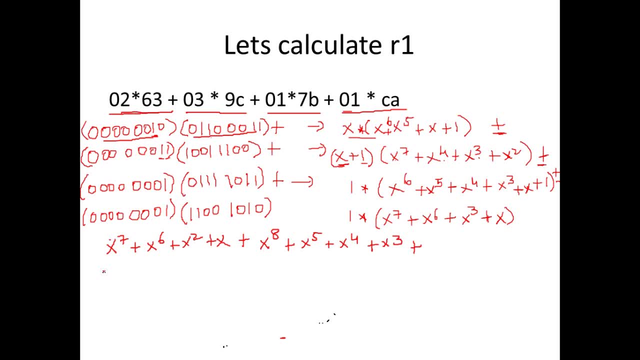 so this entire thing will repeat. so i'll write it here. that is nothing but x power 7 plus x power 4 plus x power 3 plus x square. so we have a plus here. so that is this plus, and 1 into this is nothing but the same term. so we'll write this term: x power 6 plus. 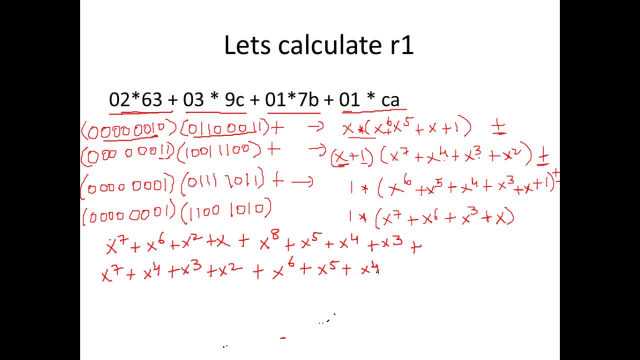 x power 5 plus x power 4 plus x power 3 plus x plus 1. so this term has come. next we have a plus, and this is 1 into this term, so this term will repeat. so that is x power 7 plus x power 6. 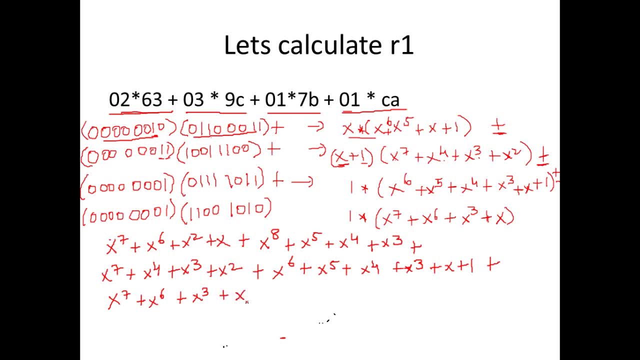 plus업 plus x, power 3 plus x. so we finish multiplying all these polynomials. so we know in finite field arithmetic two similar terms will cancel out each other. so we'll use that, say x 7 will cancel out with another x 7. likewise this x 6 will cancel out. 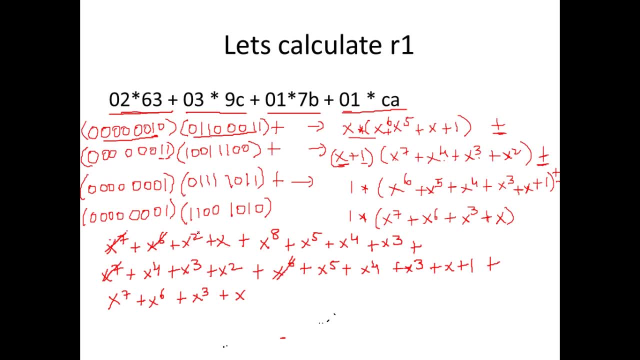 with another x 6 and x square will cancel out with another x square and x can cancel out with another x. x power 8. we don't have another x for 8, so this will remain. x power 5 can cancel out with another x power 5. x power 4 can cancel out with another x power 4 and x power. 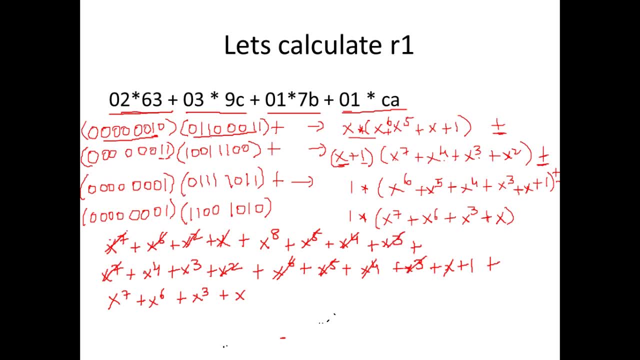 3 can cancel out with this x power 3 and you have an x power 4 here. you don't have any other x 4 4 to cancer, whereas an x power 3 can cancel out with this x for 3 and you have a 1. there is no. 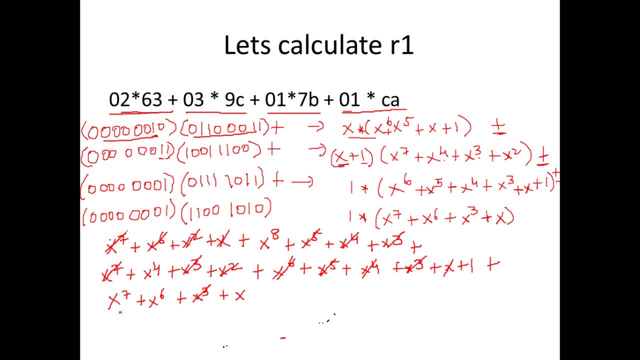 other 1 to cancel out. we have an x power 7. there is no other x power seven. x power six. there is another x for six to cancel out, again x. so what is the remaining here is this is the answer, that is, x power 8 plus x power seven plus x power six. and do we have an x power five? we don't have an. explodedeme. so we will just write what we have very good, because what we write over here that can get fewer terms. this is what is the function we're wanting. So you call that報導, we would flexibility products b. when it returns x, 3 is the field, you would write a Matsringer theme. So, as I layer, 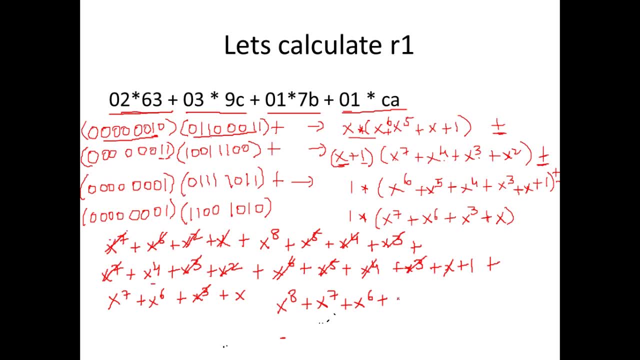 power 5. do we have an x power 4? yes, we have an x power 4 plus. is there an x power 3? there is no x power 3, x square, there is no x square, but we have an x, so we have an x and we have a 1.. 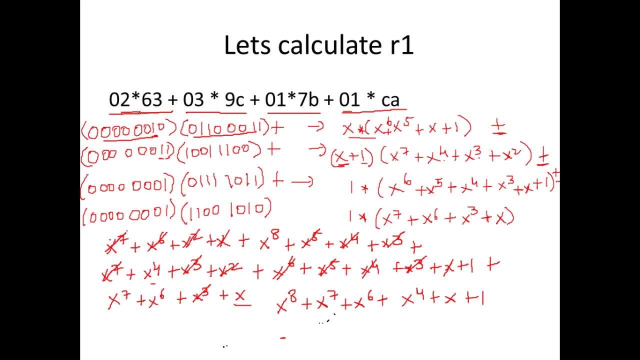 so this is the result of the multiplication and addition. the polynomial we are getting is this: in advanced encryption standard. what is the galois field we are taking? it is gf 2, power 8. so all the polynomials should be within the range. what is the range? it starts from the term 0. 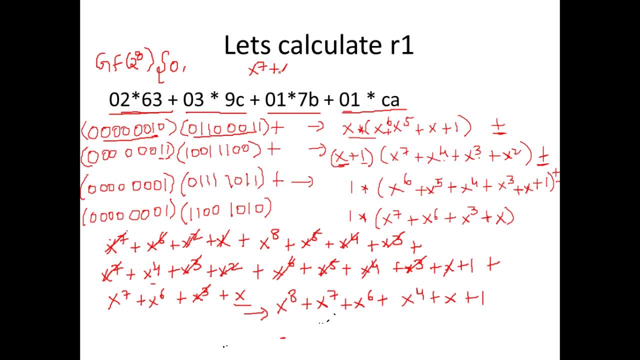 and it goes up till x power 7 plus x power 6 plus x power 5 plus x power 3. i mean x power 4 plus x power 3 plus x square plus 1. so this is the range, all the 256 elements. it starts from 000. 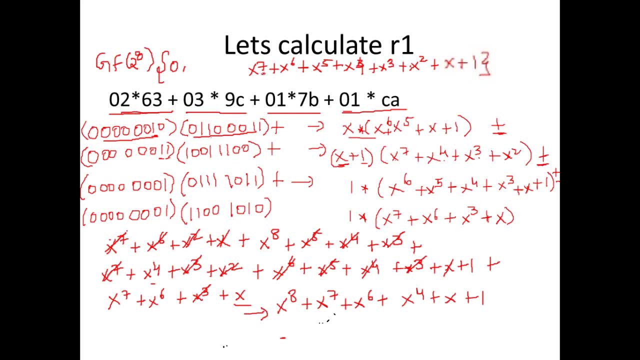 to all ones, right. so the is degree here is 7, whereas when you take a result that we have obtained is: this is x power 8. so this polynomial is not present in this galois field, 2 power 8.. so when we arrive at a result like this, what we have to do is 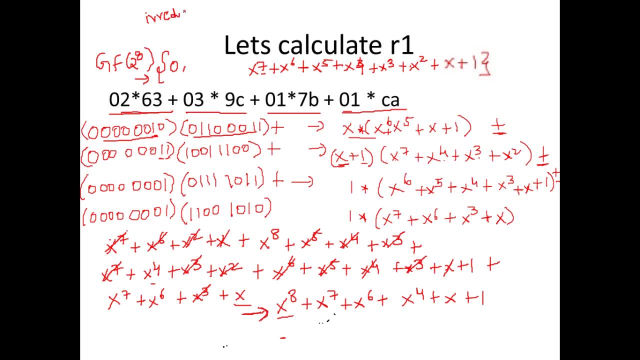 we have to use this irreducible polynomial. you know what is this irreducible polynomial? we have already seen this in galois arithmetic. so we're going to use an irreducible polynomial. divide this entire thing by this irreducible polynomial, p of x. what is this p of x? here we are going to take p of x to be. 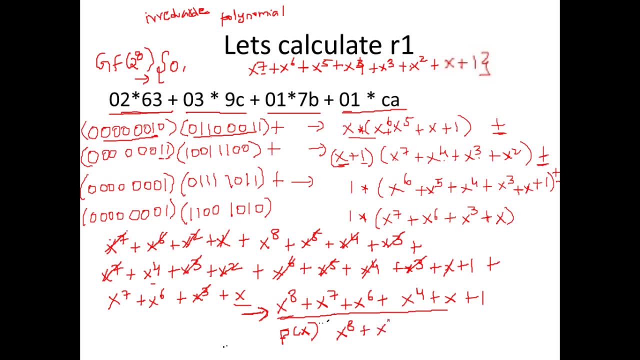 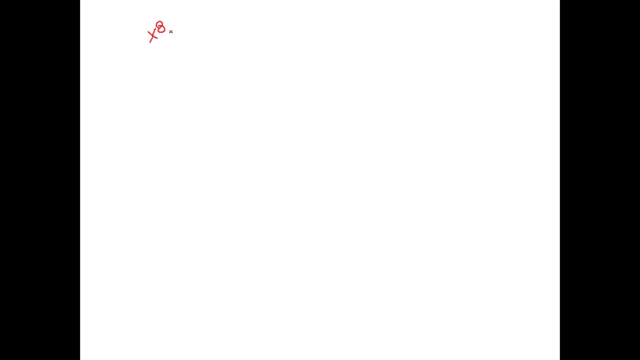 x power 8 plus x power 4 plus x power 3 plus x plus 1. so let me write it here. this is what we have: x 8 plus x power 7 plus x power 6 plus x power 4 plus x plus one. so will you represent this in binary? 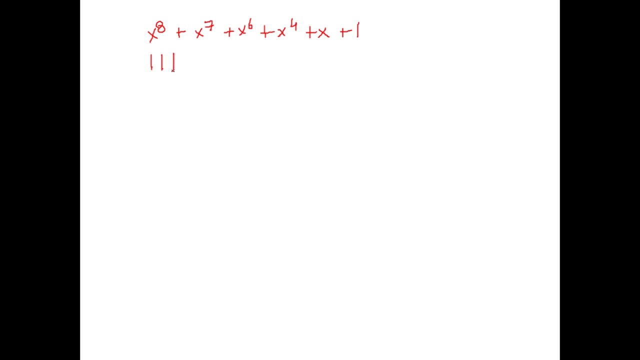 we have x power, 8 x power, 7 x power, 6, x power 5 is missing, x power 4 is there, x power 3 is missing, x power 2 is missing and we have x and we have this one. so this is the binary representation. 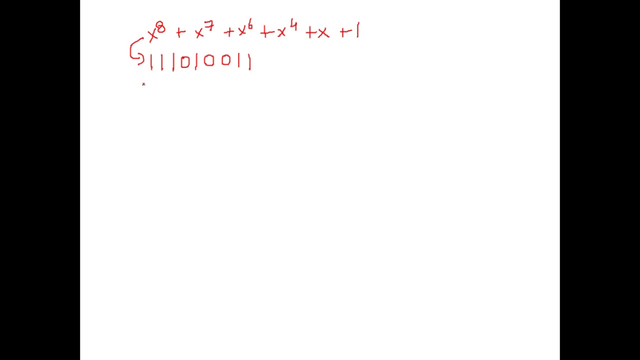 of this polynomial. likewise, we have to use this irreducible polynomial for division, right? what is that polynomial? it is x power 8 plus x power 4 plus x power 3 plus x plus 1. so what is the binary representation of this? we have x power 8, x power 7 is missing, 6 is missing, x power 5 is. 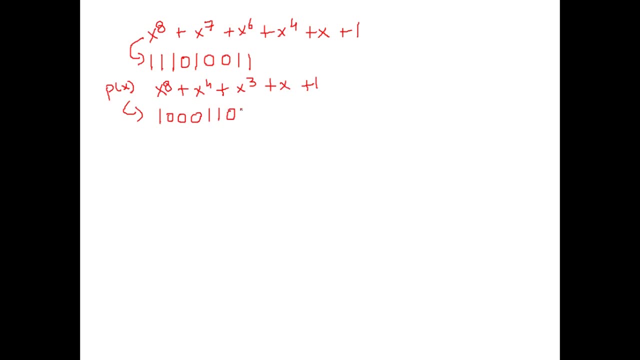 missing. we have x power, 4, x power, 3 x. square is missing x and 1.. so this is the binary representation of this polynomial. let's go and divide. let's go and divide this by this, so this division happens. you're going to take one one one, zero one, zero, zero, one one. 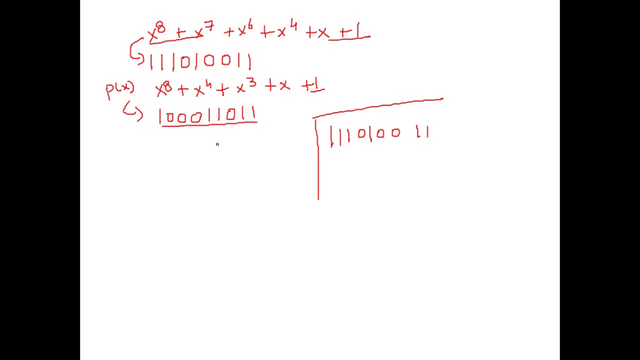 it's nothing, but we are dividing this by this, so we'll take this: 1 0 0 0, 1 1 0 1, and it's just give 1, so it's 1 0 0 0, 1 1 0, 1 1, so it's just an xor operation here. 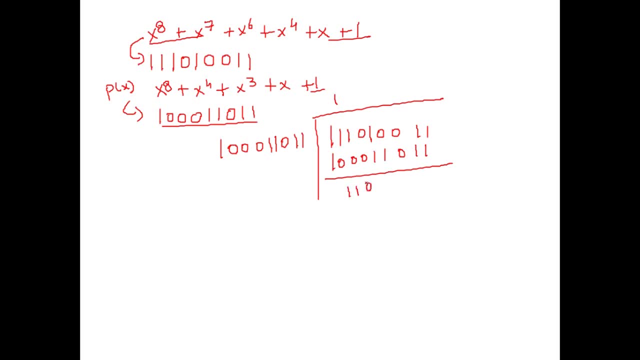 so that's it one, and one gets cancelled out. so it is one, one, zero, zero. we have one zero. these things cancel out. so this is our result. so what is one, one, zero, zero in exa? this is nothing but c. and what is one zero, zero, zero? it is eight. so we have achieved a final computation: c8. so what is the final result? that we 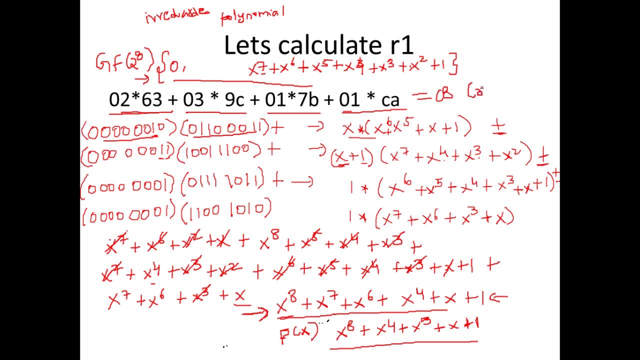 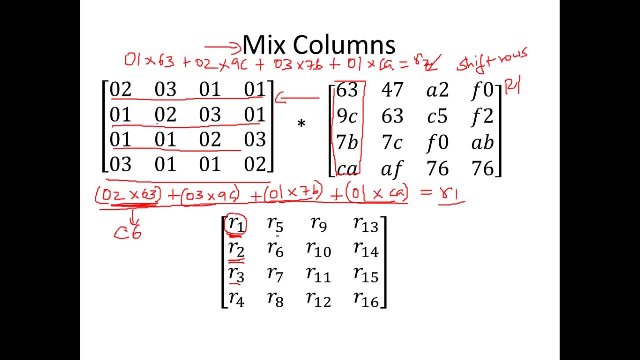 have achieved here, the result is c8, that is, nothing but r1. so going back further. so here we have achieved this computation of r1 to be c8, like that, you have to compute the entire matrix by multiplying that with this matrix. and what we are going to do here is we are going to perform everything. 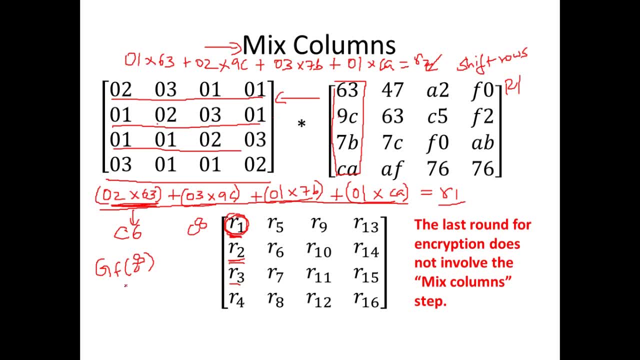 as gf 2 power 8, finite field arithmetic. if the result is a polynomial that is not present in g of 2 power 8, then what we are going to do is we are going to reduce it using the irreducible polynomial pfx. so what is the irreducible? 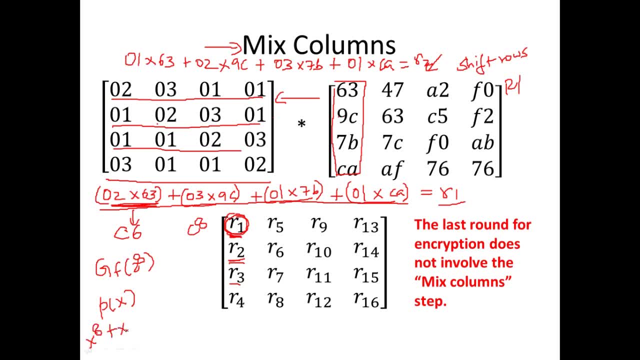 polynomial we have used. it is x power 8 plus x power 4 plus x power 3 plus x plus 1. so that is where finite field arithmetic comes in advanced encryption standard. and now you would have understood that finite field arithmetic plays a very important role in arriving at the 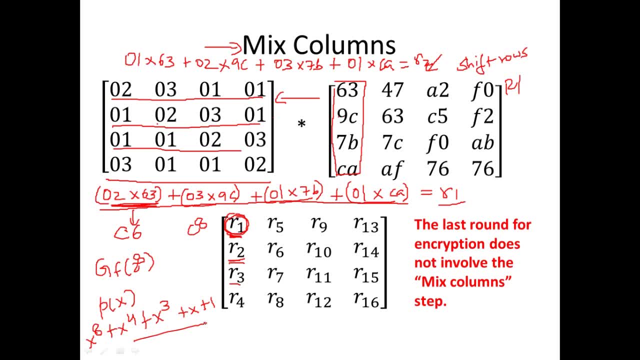 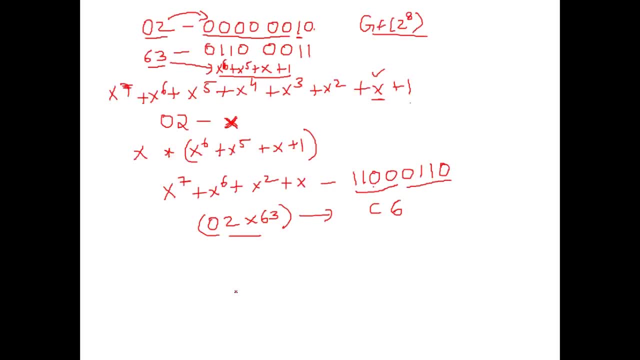 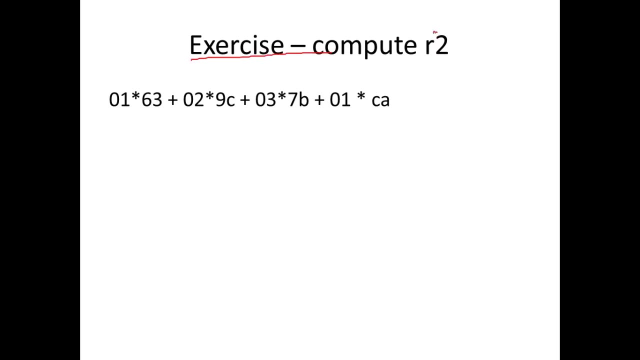 ciphertext so you can take an exercise. you can write a, you can compute r2 so you can use finite field arithmetic and you can use the strategy i have told you: compute the value of r2. if you get a polynomial of a greater degree, reduce it using the 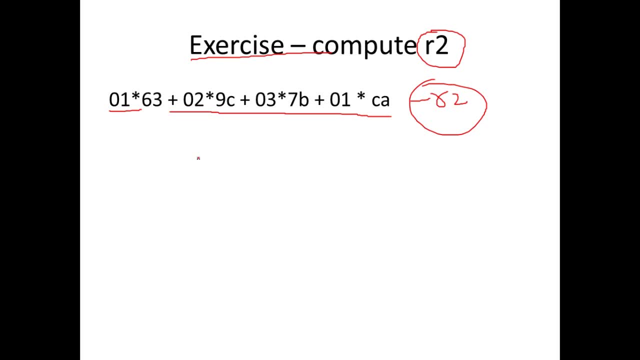 irreducible polynomial that i have given you. so this is going to be your exercise. you're going to solve this. let's say, after the mixed column step is done, we get this resultant matrix: r1, r2, r3. let's say, all our computation is done. 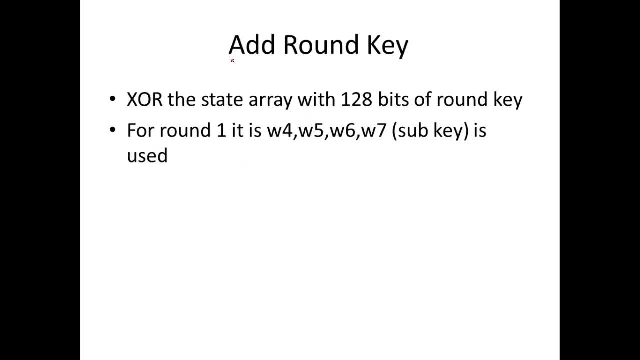 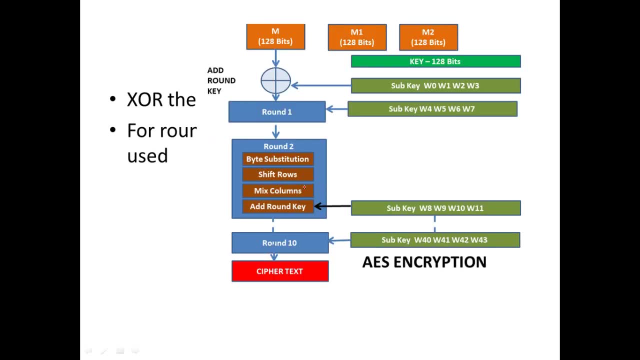 we get the resultant matrix. so what is the final step in our round? that is add round key. so what we are going to do is we are going to finish the mixed column, so we are going to get an output from the mixed columns. right, what is that? that is nothing but. 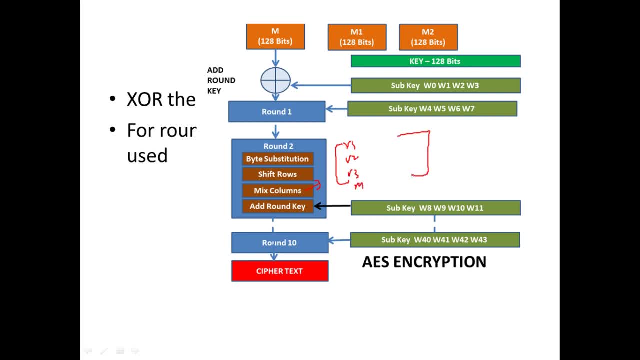 r1, r2, r3, r4. so you're going to get this 4 cross 4 matrix, which will be given to the round key and we will be performing an xr with the round key, that is, w8, w9, w10 and w11. 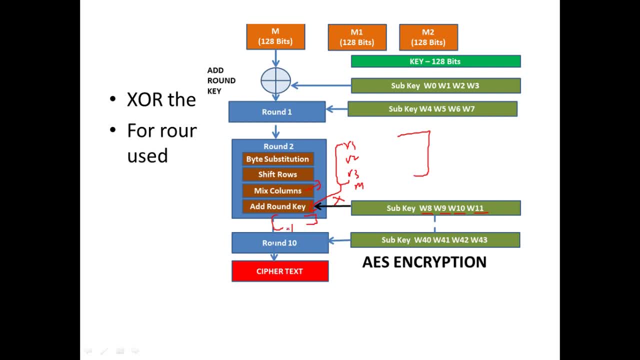 so that we'll get another 4 cross, 4 matrix, which will be given as an input to round 10. for the next round, see, in round 10 you don't have this mixed column step, so finally, the output of round 10 will be your. 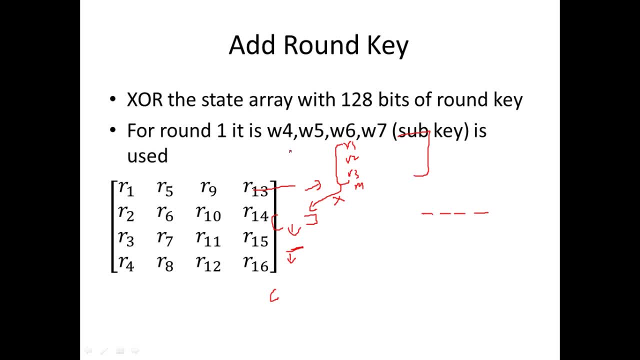 cipher text. so this is what i'm explaining you. so this is the output of a mixed column. say you have computed values, all, all values. r1 to r16 will give you 2 of n absolutes. r48 Will nuts be given to your next you go to the endtherapistcom. you choose the. 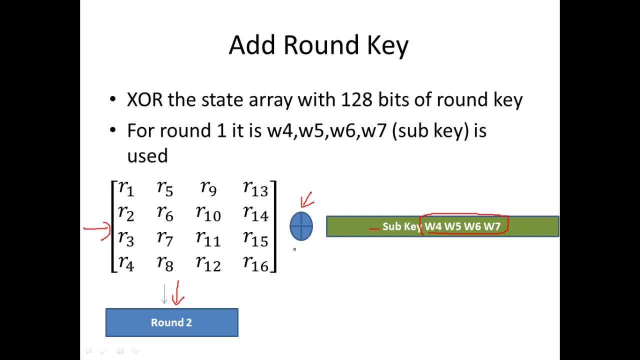 field. so that will give this stitchum for this conversion: int j1, row 8, r0, Col-0.08. then we will need x gotten w9 and i got iload 0.아니n and we will then end cipher from instant combination to 10, since we are in창 16.0. we have taken word 4 to war 7. we is along, i'll perform a next our operation and finally we'll get the output. that output we'll go to round 2 like this: that output will go to round 2 like this: willlympics 10, roms. and in the 10th round we don't have this mixed column step- and the output of the tenth round will be the ciphertext. 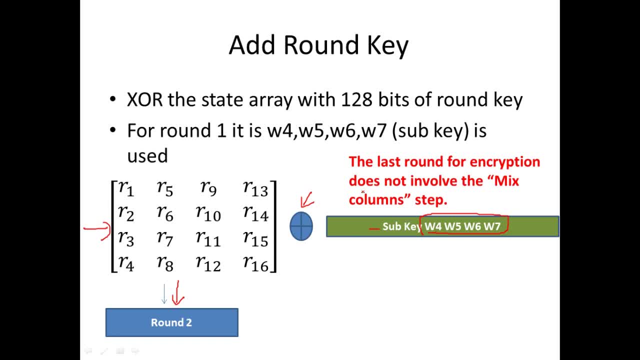 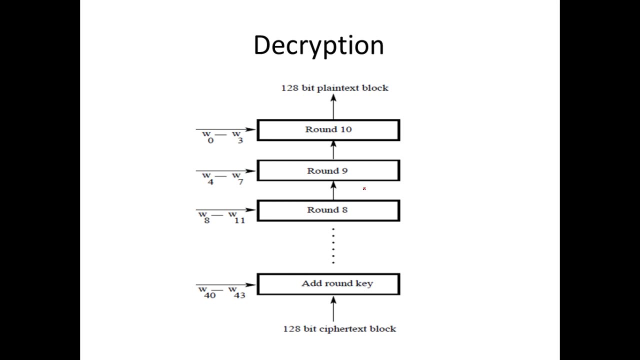 and all the multiplication and arithmetic here follows the G of 2 power 8, finite field arithmetic. now let us take a brief look at the decryption. decryption is the reverse of encryption. so what we are going to do here is we are going to take this 128-bit ciphertext block that we have arrived. 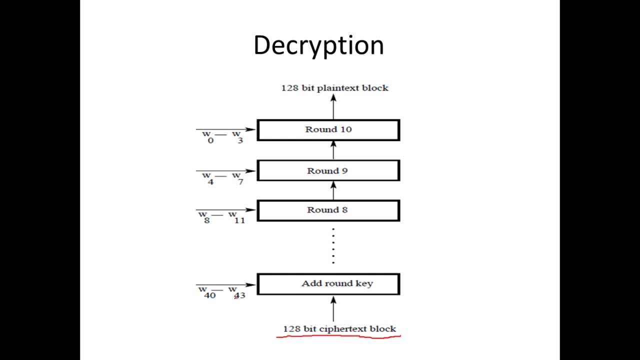 at and we'll be adding the round key, that is, we'll use the round keys in the reverse. we'll start from word 40 to word 43. we'll pass that. we'll perform an XOR here. it's a simple XOR operation with the ciphertext and this will lead to a state array, a 16 byte state array, so we'll have 16 elements here. 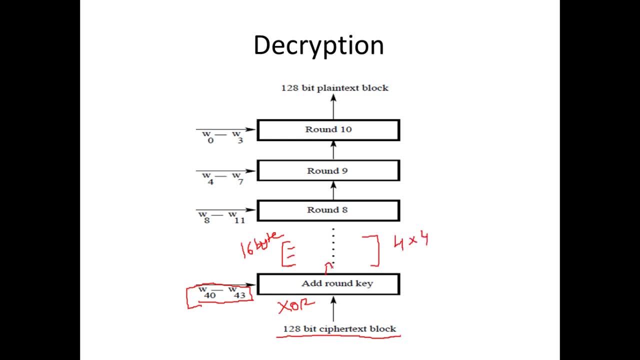 in this 4 cross 4 matrix. that will be the output of this and we'll be going with a rounds here again. we'll start from round 1 to round 10. so this output will be given to round 1 and for round 1 we. 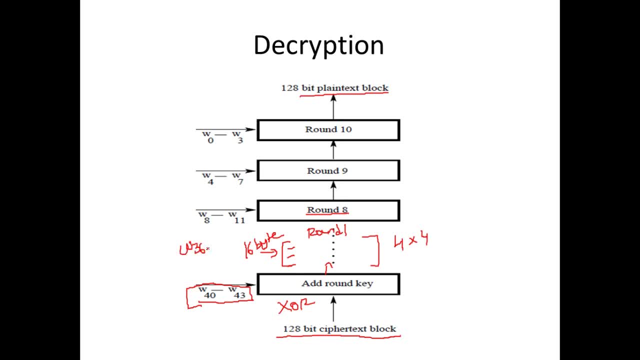 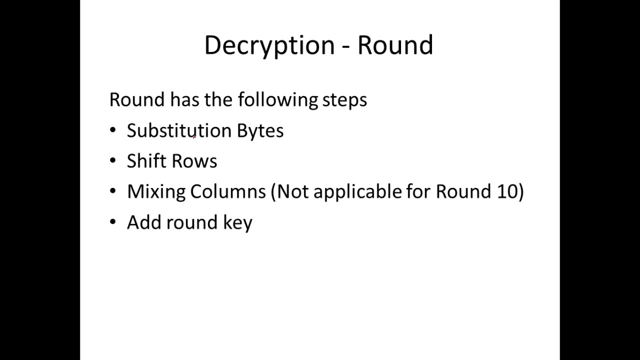 are going to use the key starting from w36 to w39. these four words will be used in round 1 and again in round 1. we have these four steps that we have seen with the encryption. let's take a brief look at the four steps we have in every round in decryption. the first thing is substitution. 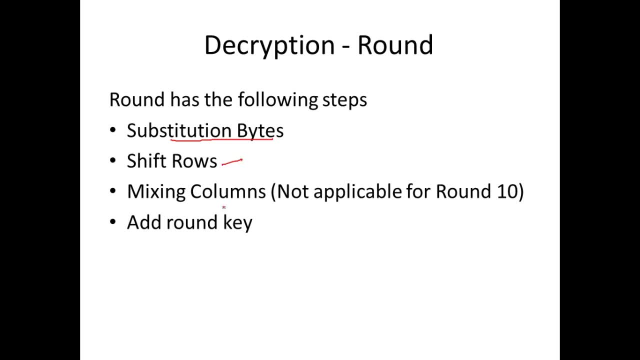 bytes, and the second thing is shift byte, and the second thing is shift byte, and the second thing is shift rows, and the third thing is mixed columns- and mixing columns is not applicable for the last round, round 10- and add round key. so we'll just take a brief look at these steps and wind up. 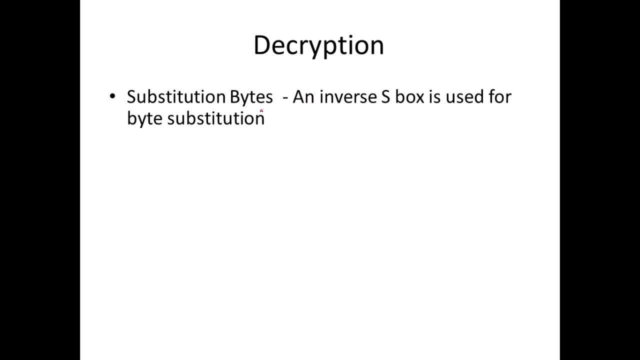 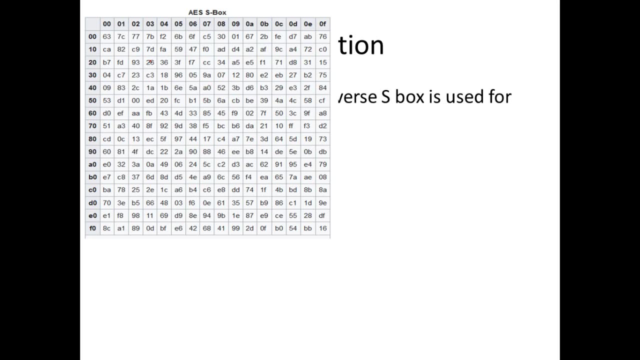 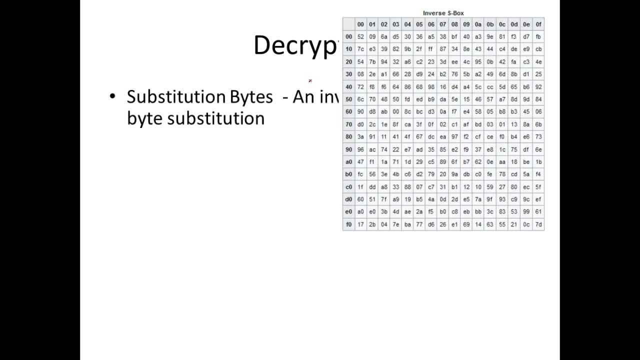 so what is substitution bytes? you remember what we did in encryption: we use this xbox for taking every byte from the matrix. we substituted that with another byte, whereas in decryption, again, we are going to do the same thing, but we use an inverse xbox. so we take every byte from the input state array. we are going to just substitute that with this. 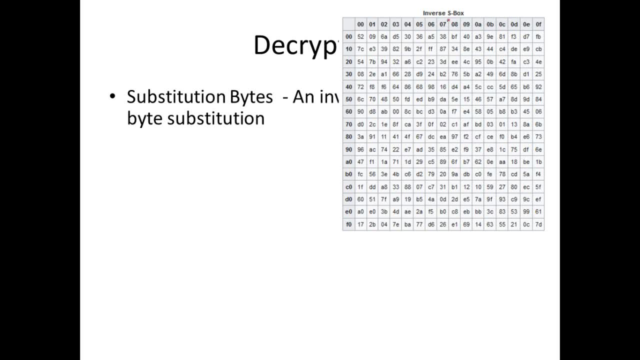 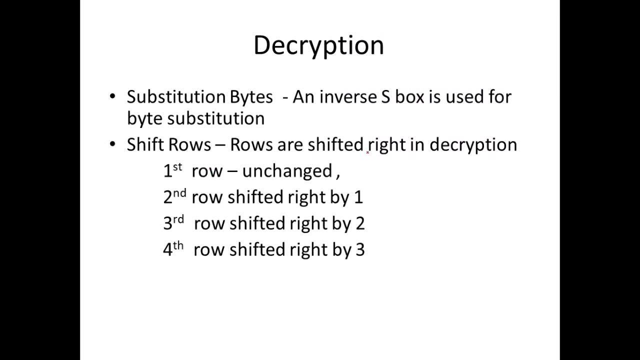 inverse s box. again the same kind of a concept. here it is an inverse s box. is used shift rows. we are going to shift rows, but here shifting will be a right circular shift. in encryption we are doing a left circular shift by one byte, two byte and three bytes, whereas here we 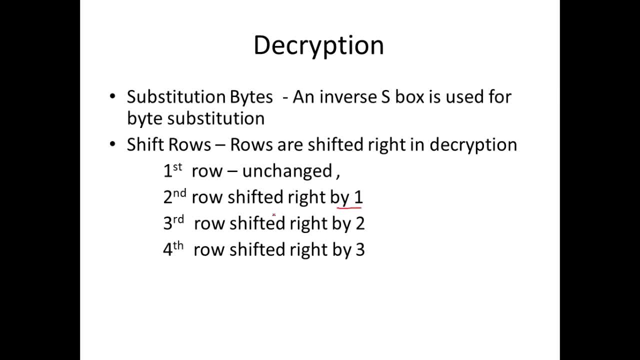 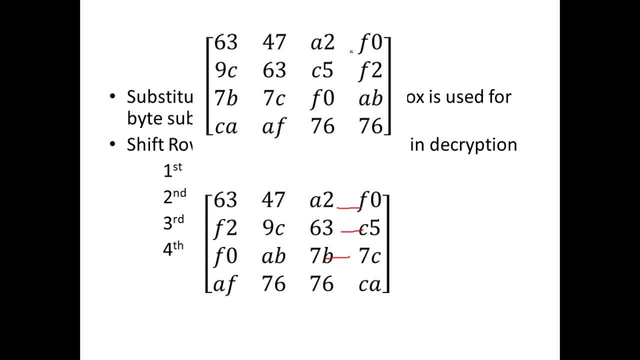 are going to do a right circular shift by one byte for row second, two bytes for row three and three bytes for row four. so if this is the input, the first row, we are not going to change anything. it's going to be like that, whereas the second row, we're going to do a right circular shift. that is, we're. 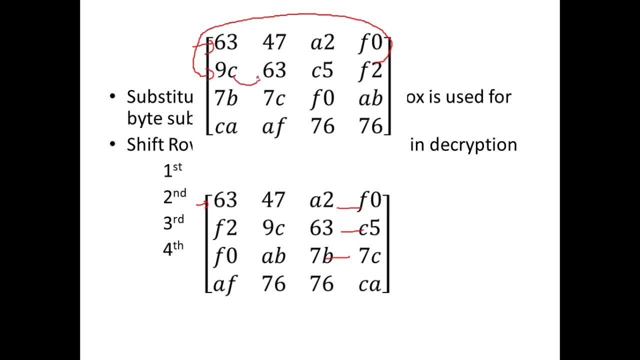 going to bring this to the front and push everything to the left by one byte. so you see f2 is here. 9c, 63 m, c5. we're going to do a right circular shift by two by. so we're going to bring ab if 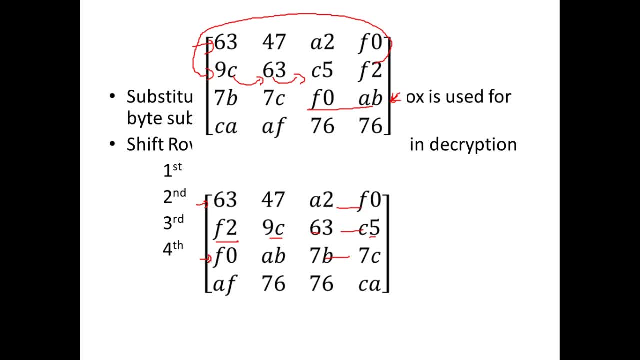 0 AB will be in the front, 7 B and 7 C will be pushed to the end. likewise, we take three elements, we push it to the front and CA will be coming to the end. just the opposite of what you did in encryption. is that clear? 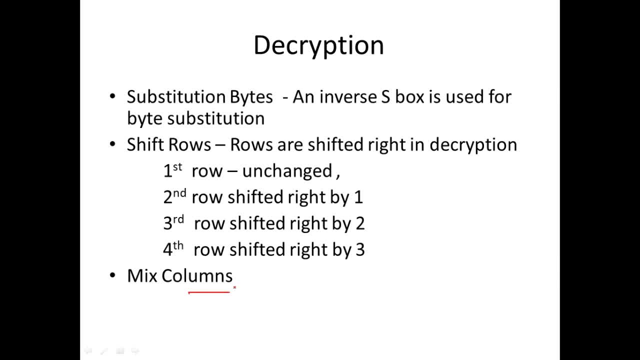 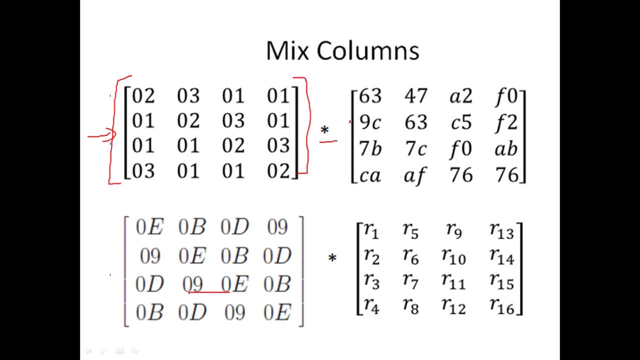 after shift rows we have mixed columns. we remember what we did in mixed columns. in encryption. we have taken this matrix, a standard matrix. we have multiplied that with the output of the shift rows state array. so now in decryption we are going to take this matrix and we are going to apply and we are going to. 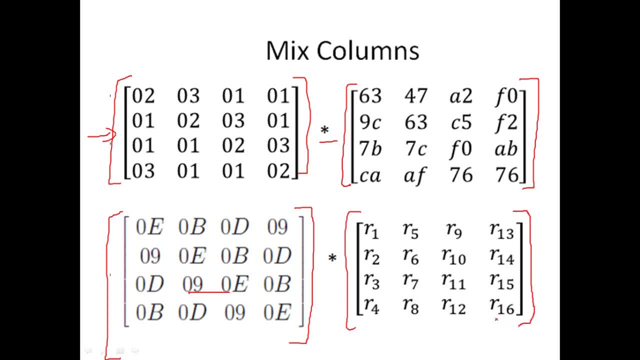 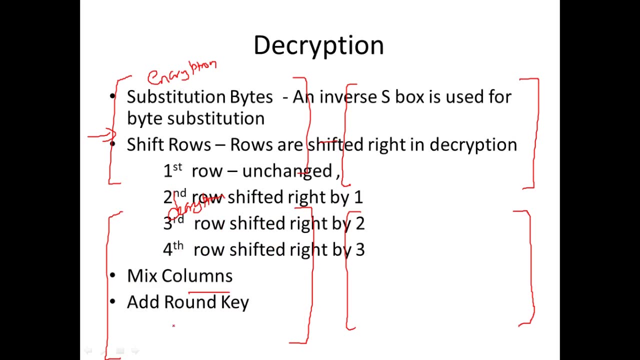 multiply that with the output of the shift rows phase. so this is for encryption, you do this for encryption, you do this for decryption. finally, add round key. so this is nothing, but the output of this step will be: you know, we'll be taking the input round key. say, for instance, w36 to w39. the word we are 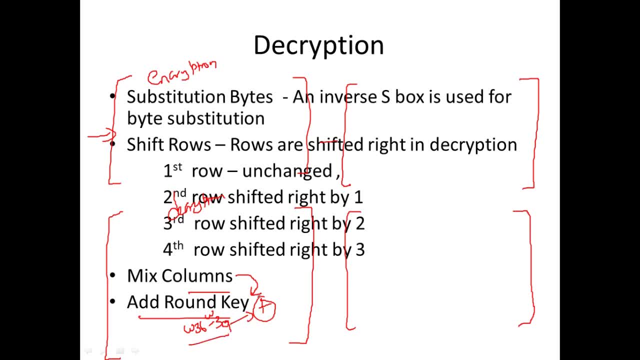 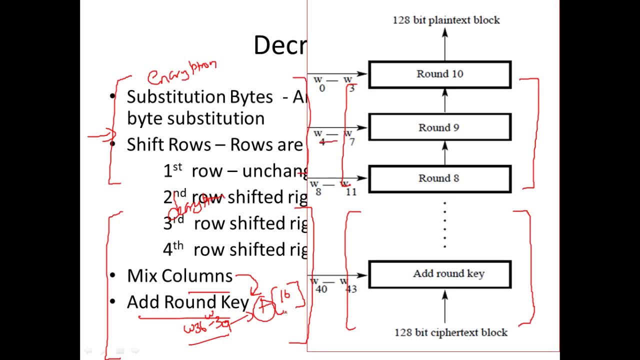 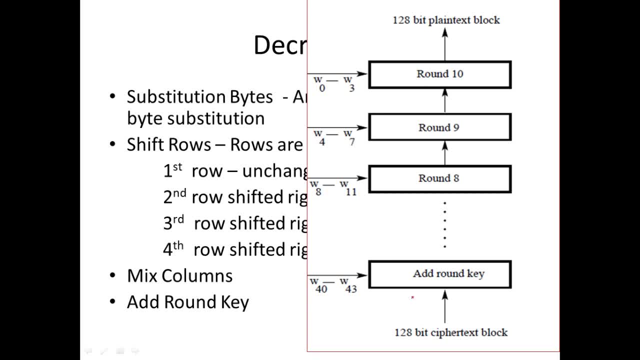